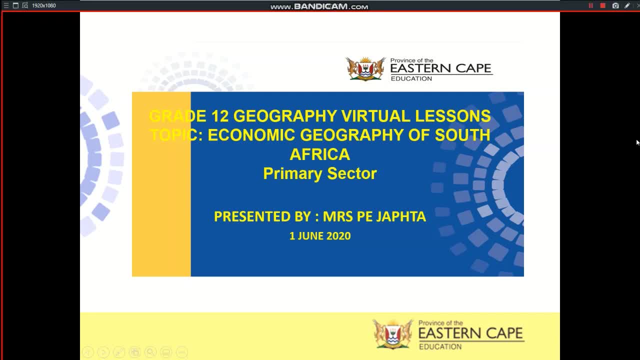 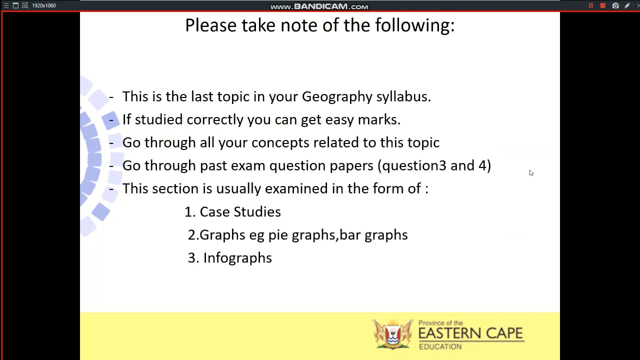 Good morning straight to our geography learners. Today we will be starting off with the last segment or last topic in your geography syllabus, namely Economic Geography of South Africa, And we will be looking at the primary sector, specifically looking at agriculture. Now you need to please once again take note of the following: This is the last topic in your geography syllabus. If it is studied correctly, you can get very easy marks. You need to go through all your concepts related to this topic. 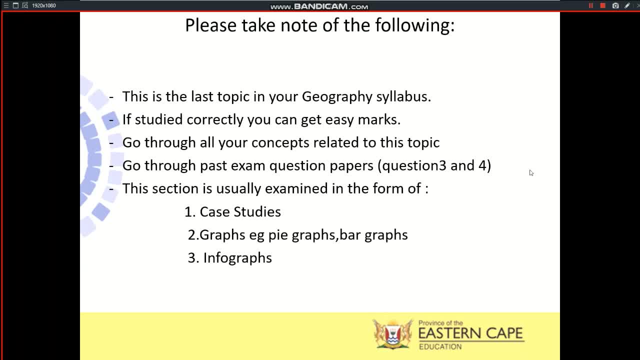 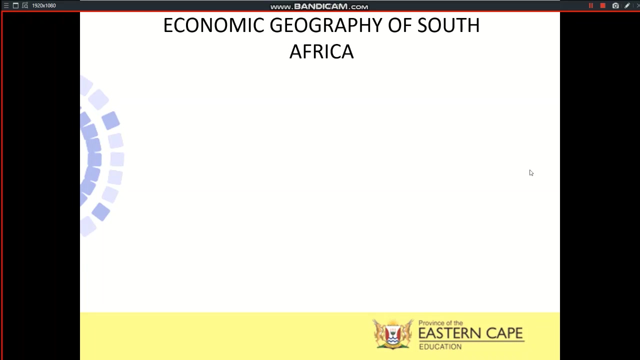 Okay, question 3 and question 4.. This section is usually examined in the form of case studies graphs, pie graphs, bar graphs and infographs. Let us find out what exactly is it in terms of what we will be studying under the Economic Geography of South Africa. 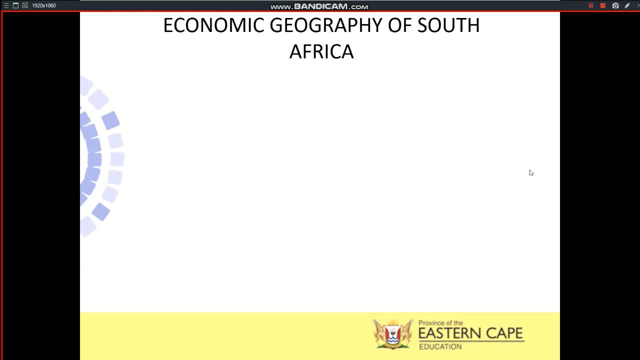 What is the economy of a country? What do we refer to or what do we understand by the economy of a country? It is as follows: The economy is a system of activities and people depending on each other to supply their needs, And that is the essence of what we will be going through. 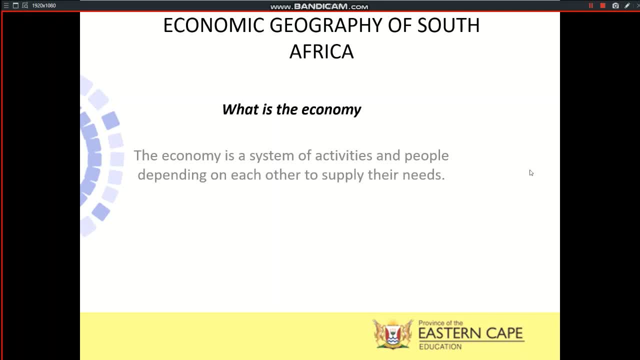 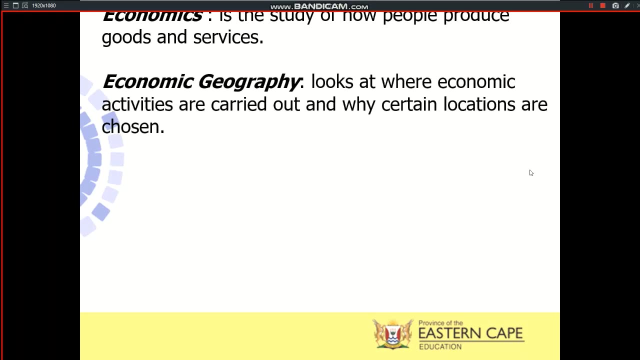 Economy is the structure of society and the economy is the structure of society. When we do Economics- geography of South Africa, Economics- what does economics mean? It is the study of how people produce goods and services. Economic geography: We look at where economic activities are carried out and why certain locations are chosen. 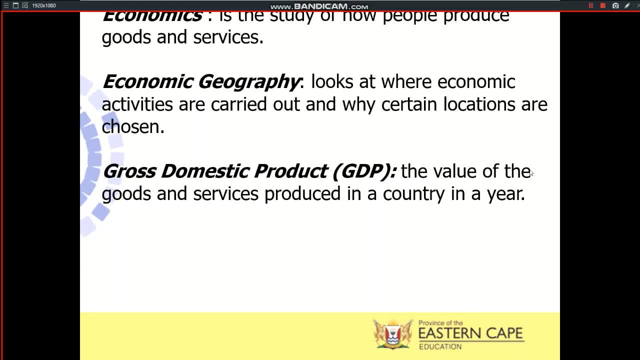 We look at a term called Gross Domestic Product, GDP, which is a common term or a common concept that you will be coming across in each of the sections of this topic, so you need to know it. It is the value of goods and services produced in a country. 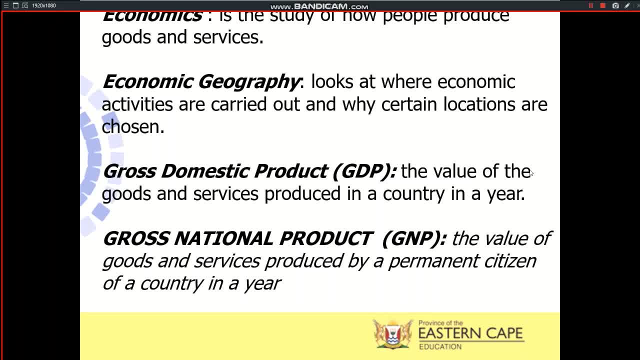 The gross national product. the GNP is the value of goods and services produced by a permanent citizen of a country. Now, learners, these are just some of the concepts that you need to know under the economic geography of South Africa. You need to go once again, go to your textbook, go to all the other concepts and go through them and see that you know them very well. 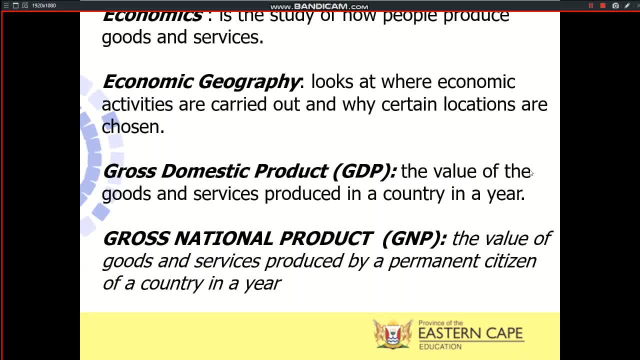 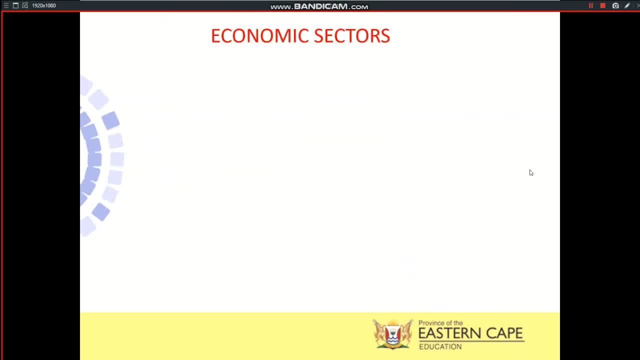 Again, it is very easy to score marks if you know these concepts. Let us look at the economic sectors in our country, In other words, the sectors that contribute to the economy of our country. Let's look at them, And these sectors are very important. 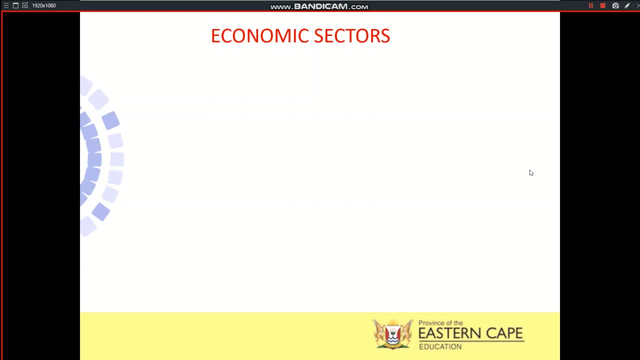 You must know them. You actually also study, or some of these sectors are also referred to in other subjects that you are doing. So it is not only in geography that you do it, it also comes up in some of your other subjects. Let's look at the primary sector. 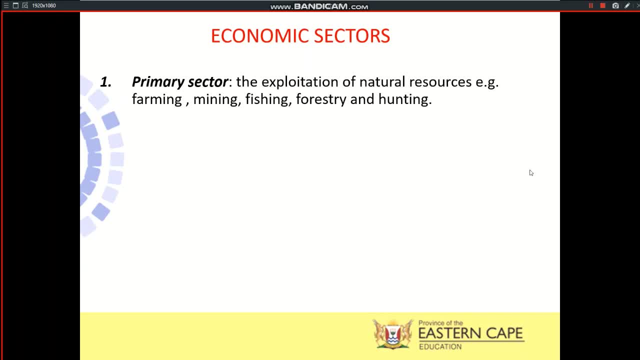 And we have already referred to them. When we did settlement geography, we referred to some of them. The primary sector: This sector refers to the exploitation of natural resources, In other words, farming, mining, fishing, forestry and hunting- Everything that comes from nature. 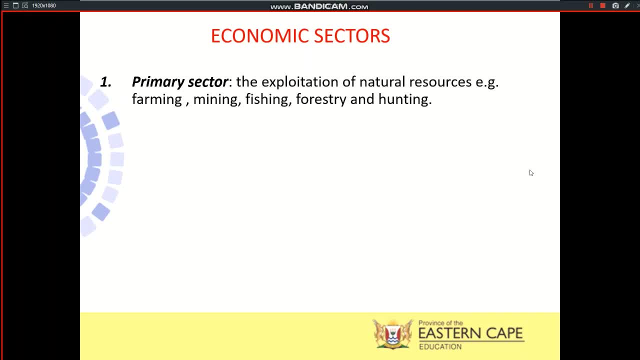 It is the primary sector When people farm, mining, fishing, forestry and hunting, Just to repeat, This is called the primary sector. Let's look at the secondary sector. Secondary sector, where raw materials are changed into something more useful and valuable. 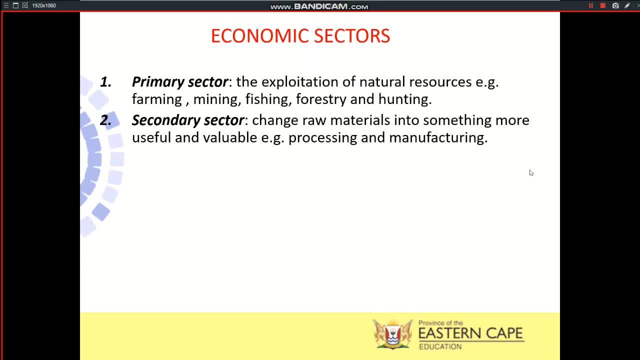 In other words the processing and manufacturing industry, Where people are processing and manufacturing goods- And here we speak of light industries, heavy industries, where people manufacture goods- It is called the processing and manufacturing industry. The third sector is called the tertiary sector. 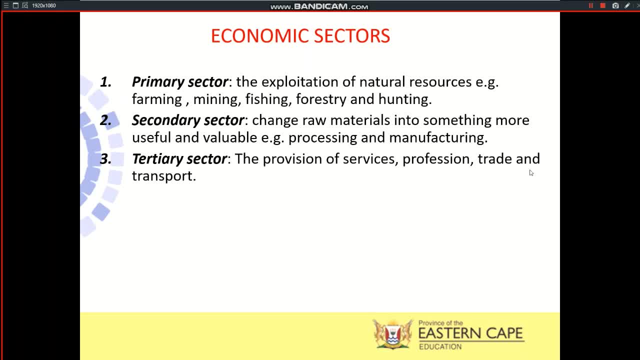 This is the provision of services, that is, professional trade and transport Where people or let us say where there is the provision of services. The fourth one is called the quaternary. Quaternary sector. This is usually the intellectual services. 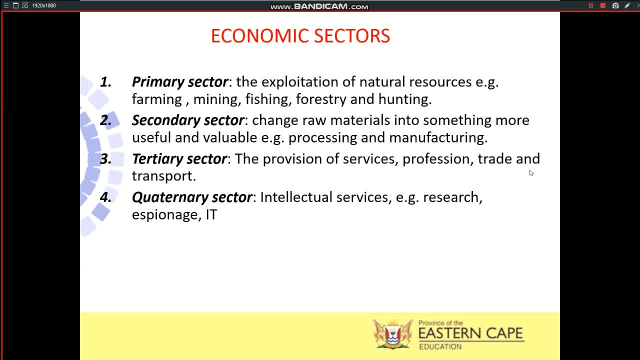 Example where research is done: IT, etc. So these four sectors, you must know They can be examined as a concept And they can examine it even referring to it as part of a question. Let's look at the following. 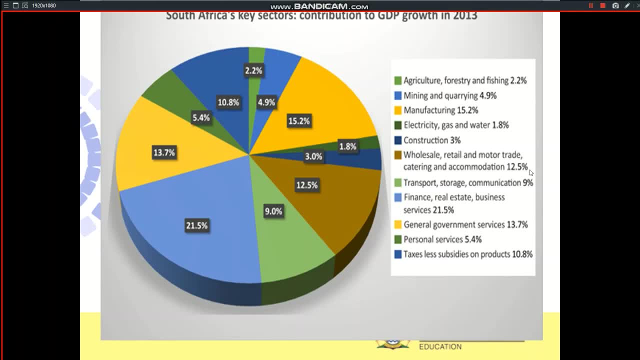 This is called South Africa's key sectors And how they contribute to the GDP growth. This was just a pie graph where they actually show you how these sectors contribute. This was contribution to the GDP, That's the gross domestic product, in 2013.. 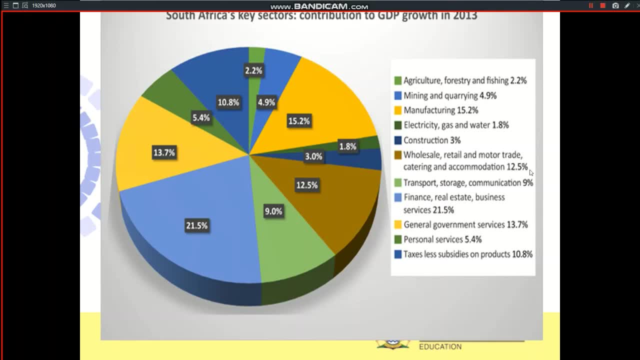 But let us just look at it. You can see they speak of agriculture, forestry and fishing- 2.2%. If you go to the graph, this is a pie graph And you can see they can ask a question from a pie graph. 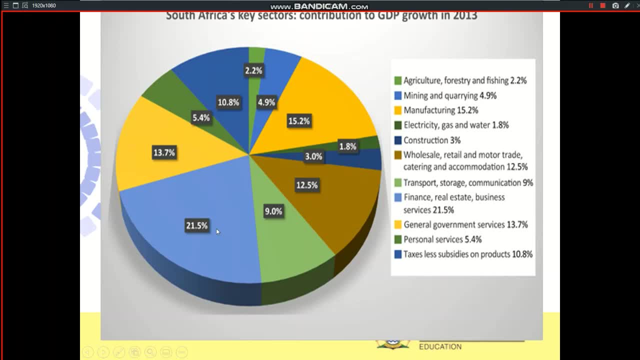 where data is given. So this is an example of a pie graph. The agricultural sector, forestry and fishing, which is primary, the primary sector In this specific year. that sector contributed 2.2% of the gross domestic product. So there you have it: 2.2.. 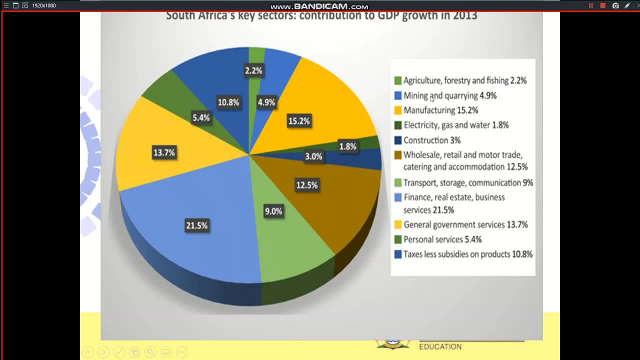 That sector over there. Then mining and quarrying. Mining is also a primary sector And this is the blue over here. That is the primary sector. Manufacturing secondary sector: 15.2%. There you can see the sector over there. 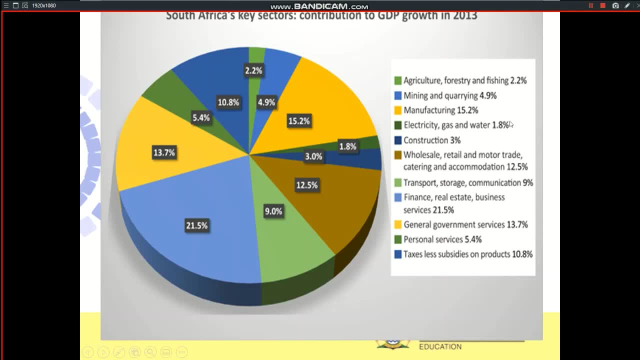 Right Electricity, gas and water, rendering of services, the green over there. Right Construction, right Wholesale and retail. there you can see secondary Transport, finance, retail, business, general government services, personal services, taxes. So in this specific graph, learners. 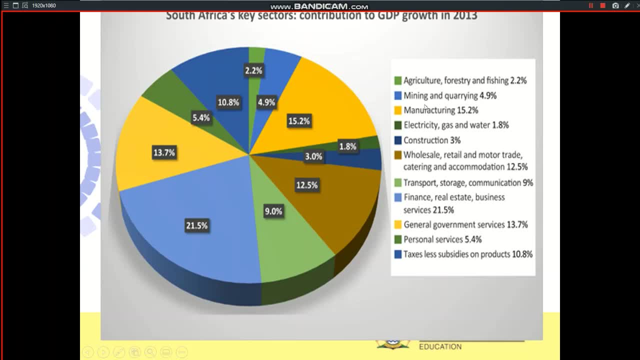 it is actually telling you what is the contribution of the various sectors to GDP. So a question can be asked on this pie graph and you can see data Here. you need to analyze the data. The data is on the graph and all you need to do is 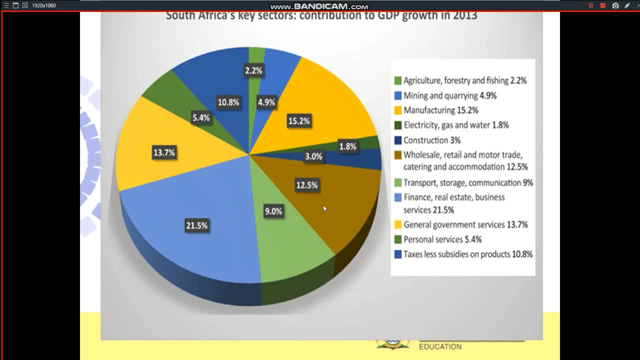 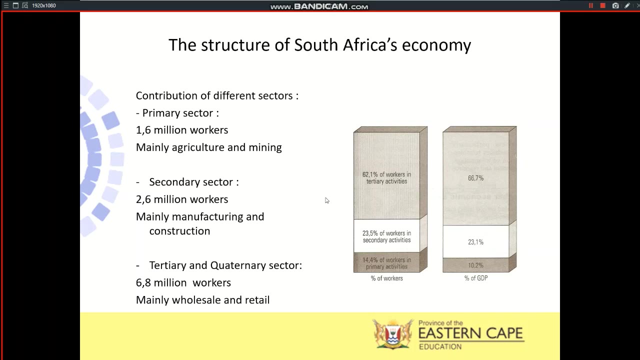 you need to look at the graph, look at the questions and see the relation between the question and the graph. So this is again one of the ways in which your questions can be answered and that you need to know. Let's go to the structure of South Africa's economy. 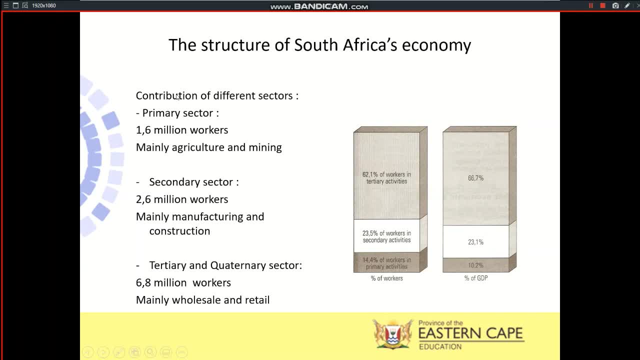 The actual structure. Let's look at the contribution of the different sectors again. Right, If you look at it, the primary sector. Right In the primary sector, how many workers basically work here? Now, this was basically just one of one particular year. 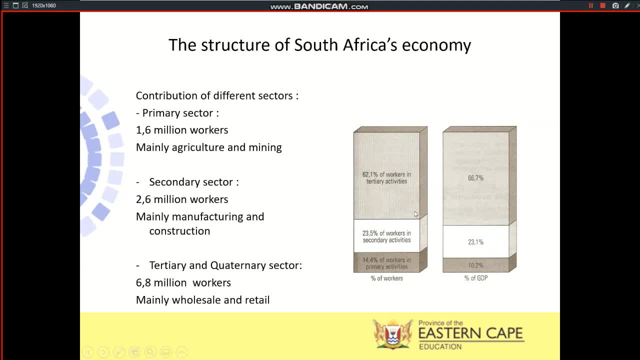 that they looked at the structure of the economy, But the idea is for you to basically just get an overview of what do we mean when we say the contribution of the different sectors. In the primary sector, 1.6 million workers work there and it's mainly in the agricultural sector. 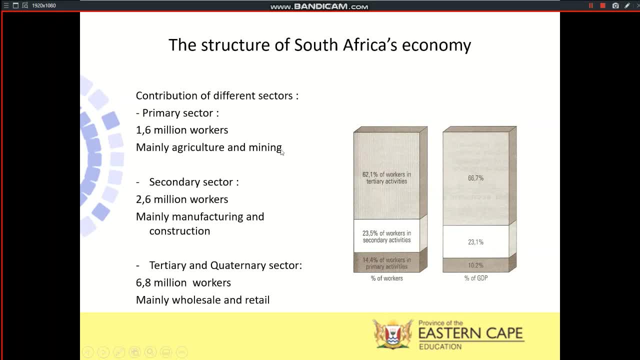 and in the mining sector Right. So when we look at our graph here you will see at the bottom of the graph right you can see the contribution, the primary sector There you are in that area. That is mainly agriculture and mining. 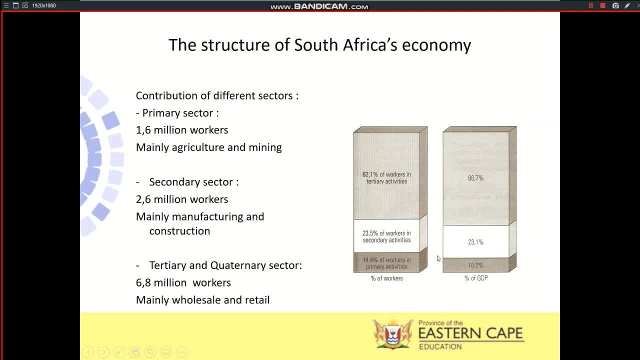 When we look at the secondary sector and the, that's the percentage of workers in the primary sector, Right, But when we look at the percentage, the contribution to the GDP is 10.2%. Then we go to the secondary sector. Here we have more workers contributing to the GDP. 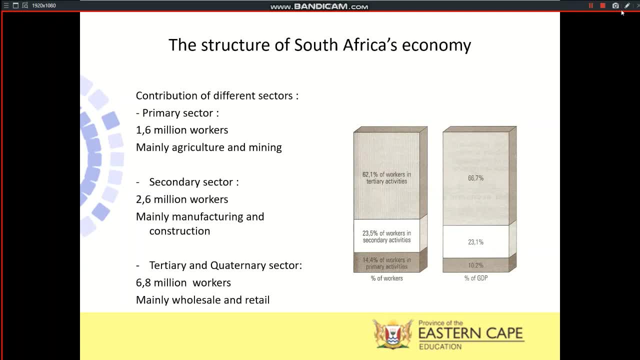 and it's mainly 2.6 million. If we go once again just look at the secondary sector, it's 2.6 million workers that contribute to the GDP and it's mainly in manufacturing and construction. If you go to the graphs over here, 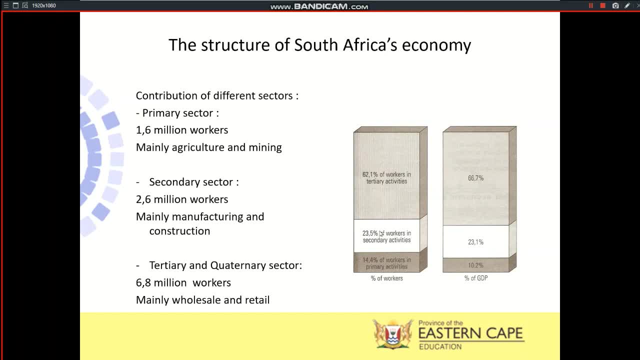 it tells you the 23.5% of workers are involved in the secondary sector and they contribute 23.1%. Then the last one, the tertiary and the quaternary sectors: 6.8 million workers, mainly wholesale and retail. 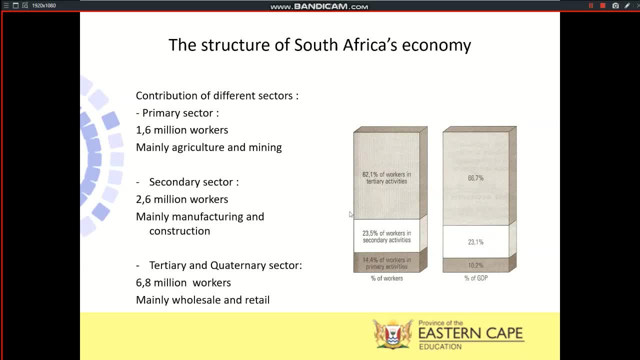 And if you go to this graph over here, you'll see 62.1% workers in the tertiary activity and it's 66.7%. that is the contribution they make to the gross domestic price. So when you look at this, you will see that as we move from the primary 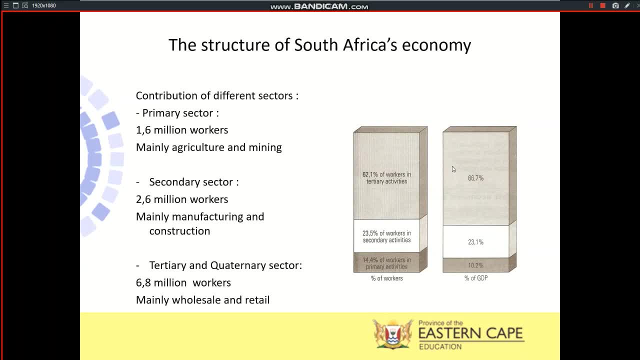 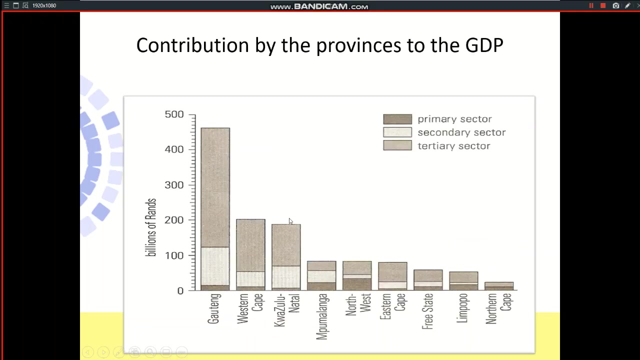 to the secondary- sorry, to the tertiary and quaternary sectors. you will see the numbers are increasing. So this is an idea to tell you how our economy is structured in South Africa. Let's look at the contribution by provinces to the gross domestic product. 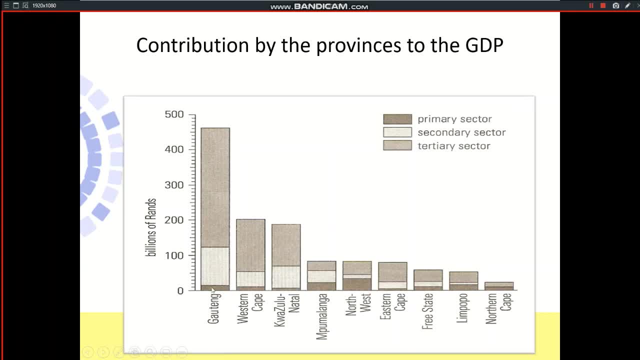 Right. In other words, this is our provinces. as you can see, all of them are here and we need to look at them individually. This is a graph to show you the contribution. Now, if you look at it, Gauteng being. 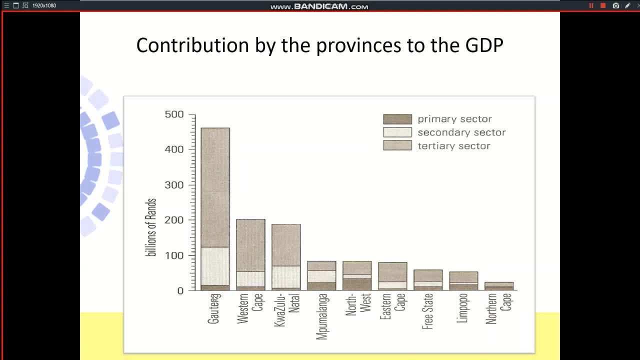 we know is the biggest province because it's the commercial hub of the country And therefore there would be a bigger contribution to the economy. Right, Look at the primary sector, look at the secondary sector and look at, most important, the tertiary sector. 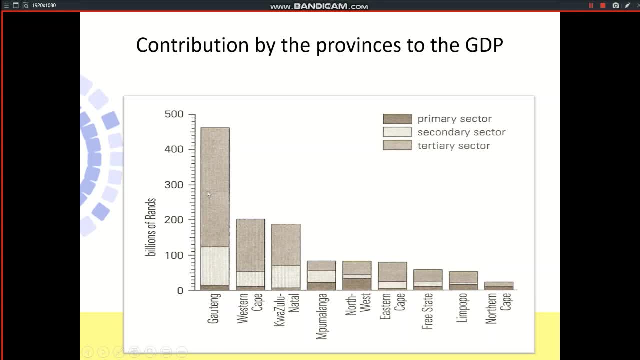 Because the tertiary and quaternary sectors in this province will be very, very high. It's the economic hub. Many people have jobs that offer very, very high quality Right And they also earn the bulk of wages very good, not wages. 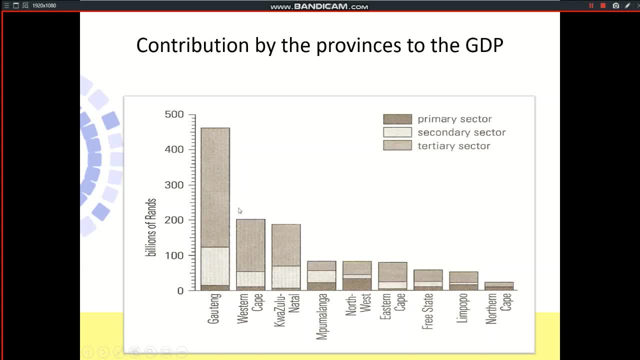 salaries that they earn in this province. The second province is Western Cape, and there you can see their contribution. KZN is the third one, And then we have Mpumalanga, Northwest Eastern Cape, Free State, Lampopo and the Northern Cape. 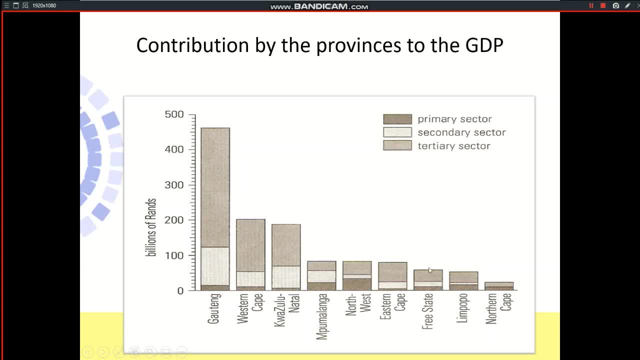 And when you go through all of these provinces, you will see by far that the tertiary sector is contributing a lot more to the GDP, And this is because, as time has gone by, the sector has increased considerably. Again, here is a graph in front of you. 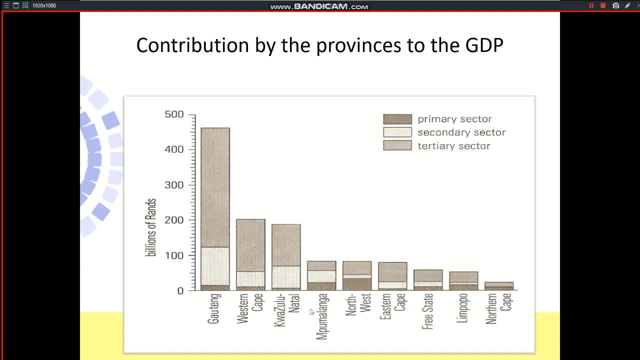 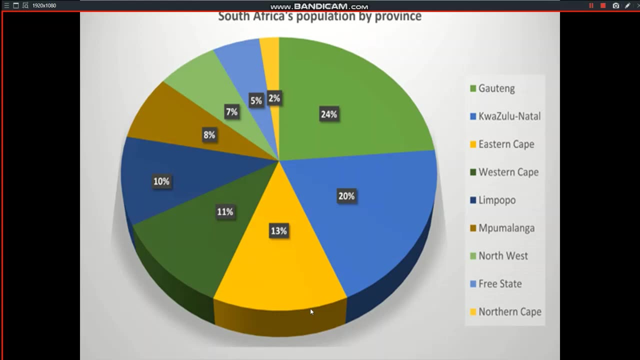 It's a bar graph, learners, And take note. they can ask. the examiners can ask, or this part can be examined using this type of graph. Here's another pie graph and this is to show our population by provinces. This is just a population graph. 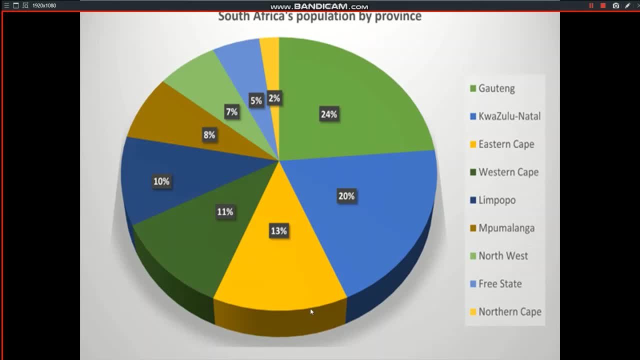 pie graph and questions can be asked on pie graphs as well. I've now showed you a bar graph, a pie graph, and this is to make you aware of basically how the different graphs are presented. Please familiarize yourself with this in this sector. 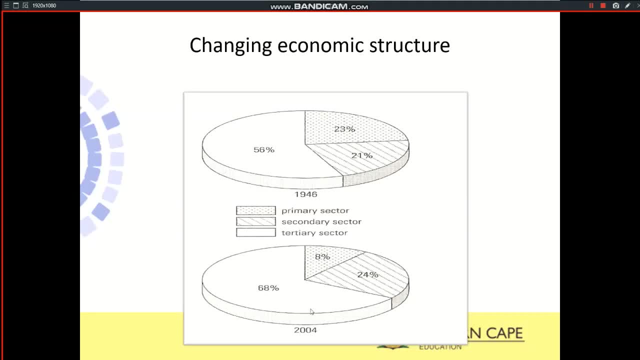 in this section Let's look at how the economic structure has changed. This is just an example to show you how the economies are changing, or how our economy has changed. In 1946, right, look at- the primary sector was at 23%. 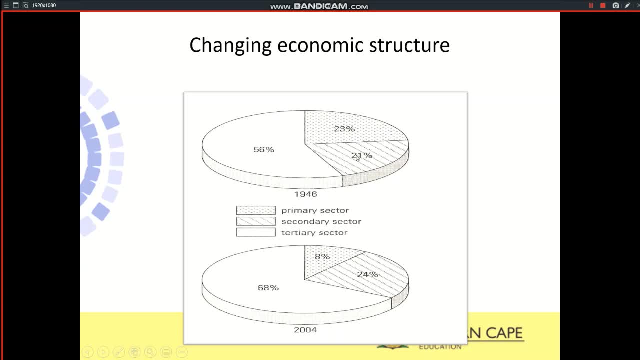 Our secondary sector was at 21%. Our tertiary sector was at 56%. But if you look at 2004, and even if you go right up to presently, this sector, the tertiary sector, has increased by far. So we will see that. 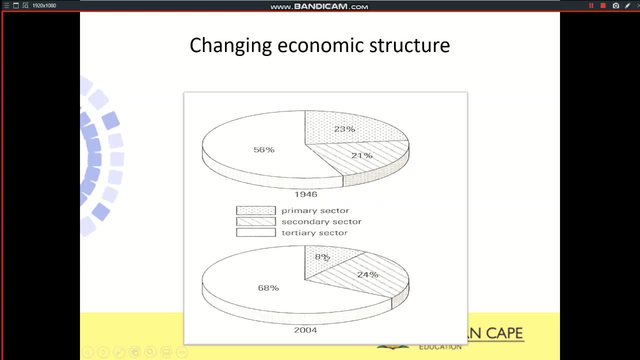 the 19, in 2004,. your agriculture, your primary sector, can you see, has decreased considerably And our, our secondary sector, has increased. This sector has decreased- And we'll find out later why- Because of the following: 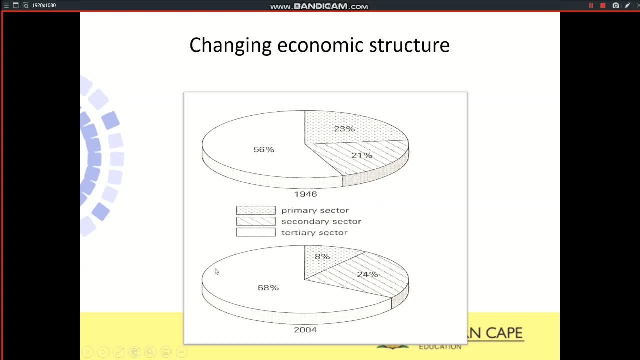 that more people are now in the tertiary sector. But as we go along with the lesson, we will explain this to you as well. Here's another way in which we've presented data here, again in the form of a pie graph. Let's look at the primary sector. 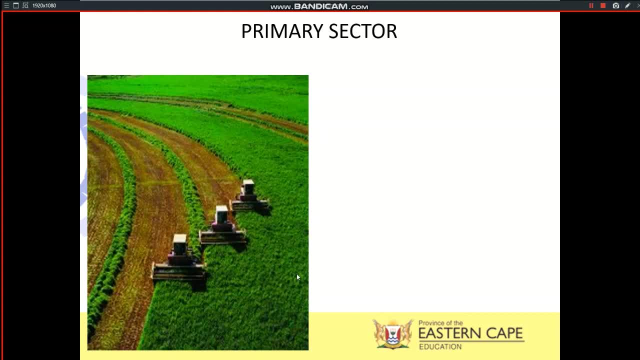 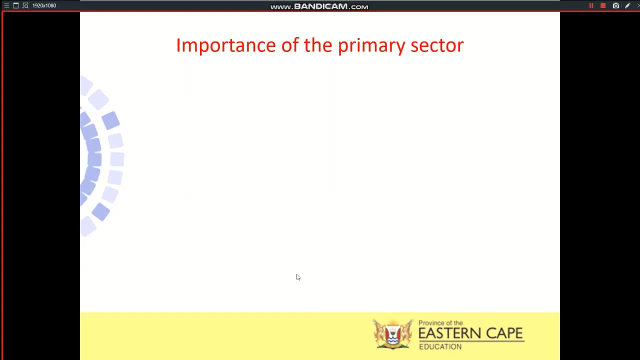 We're talking there again of farming and mining. We look at these two, My farming and mining. Let's look at the importance of the primary sector. What role do they play? It's important that we should know this. It provides food. 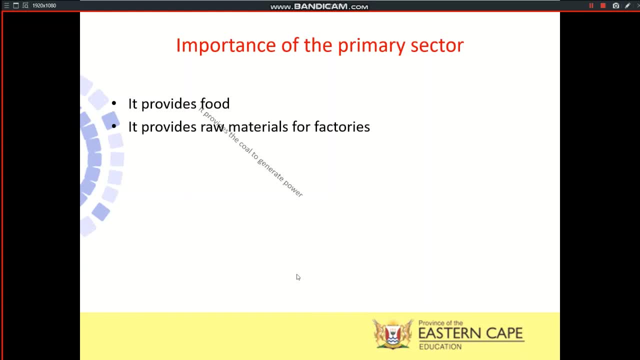 It provides raw materials for factories. It provides the coal to generate power. It provides valuable export products. It provides employment. It stimulates the development of infrastructure. It stimulates the development of industries. Let's look at agriculture, Because agriculture is one of the 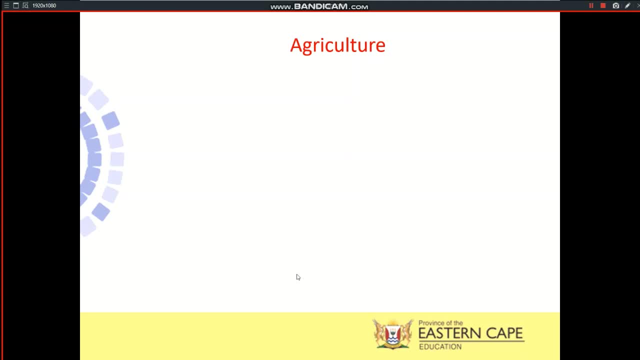 the one of the sectors that we discover that we study under the primary sector Right. Let's look at agriculture more closely and see basically what it entails. The main agricultural products in South Africa are your field crops. example: maize. We have. 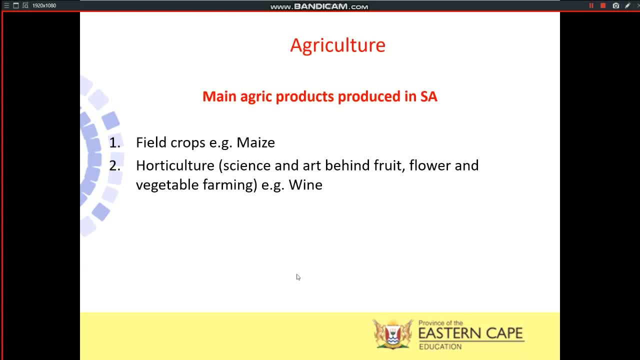 behind that science and art is behind Fruit and vegetable farming, And we've got wine as well. We've got animal products- example, your meat and wool. Let's look at farming as well here, under this product: Farming. 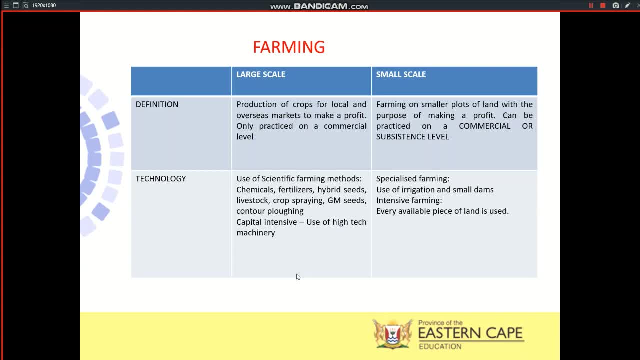 definition of farming: when we do agriculture, because we're doing farming, it is the production of goods, production of crops for local and overseas markets, to make a profit. It's only practiced on a commercial level because it's large scale. Then we have small scale farming. 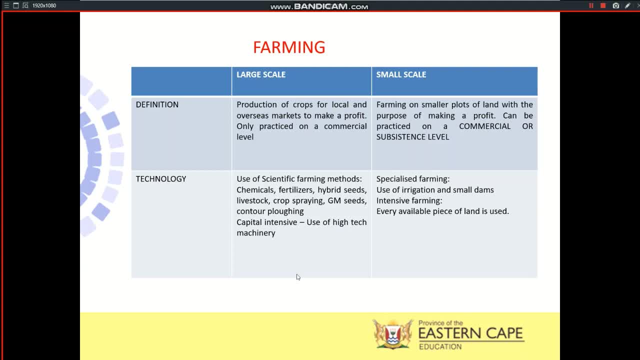 It's farming on smaller plots of land with the purpose of making a profit. It can be practiced on a commercial or subsistence level. Okay, Let us just look at these two factors: commercial or subsistence level. We will discuss them later. 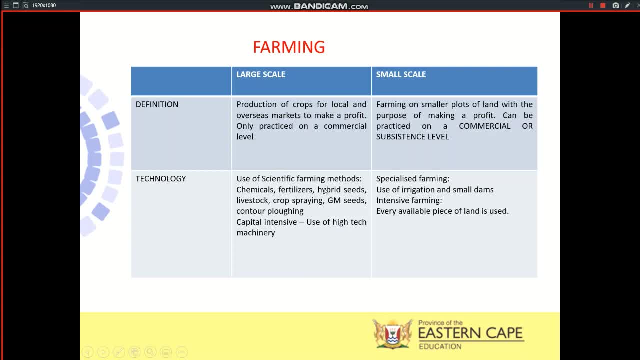 Technology. how does that contribute? In the modern era, we make use of scientific farming methods, And here we use chemicals, fertilizers, hybrid seeds, livestock crop spraying, genetically modified seeds, contour plowing, capital intensive use of high tech machinery. 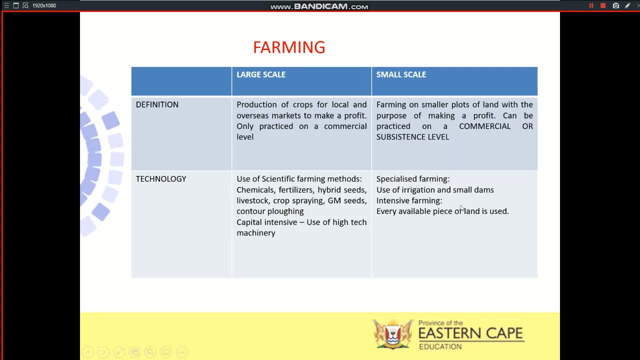 Small scale, specialized farming, use of irrigation, small dams, intensive farming- every available piece of land is used. So what we basically discussed here, people, is, when we look at farming, when we look at commercial farming, it's usually 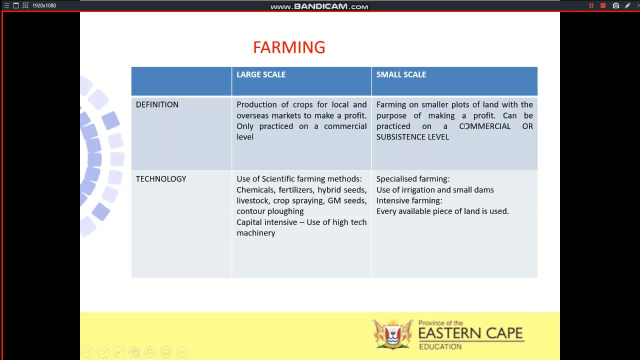 main aim is to make a profit, and it's usually practiced on a large scale, And that is why we looked at this specific column over here. large scale: This is what commercial is. farming is all about Subsistence farming is usually small scale. 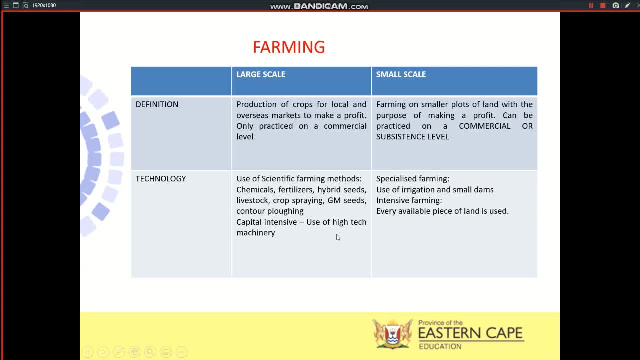 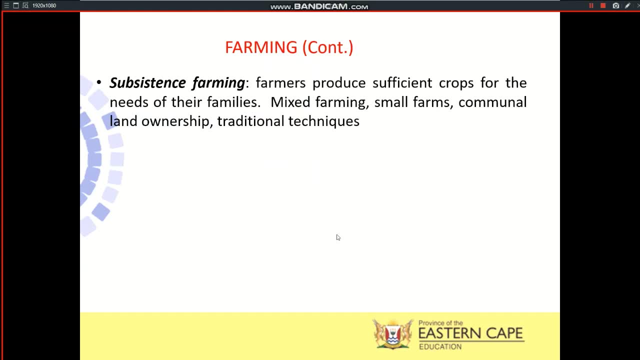 and this is basically what it entails. Then subsistence farming. let us look at it closely. It's farmers who produce sufficient crops for the needs of their families- only, Usually mixed farming, in other words, they plant a variety of crops, and that is why they use. 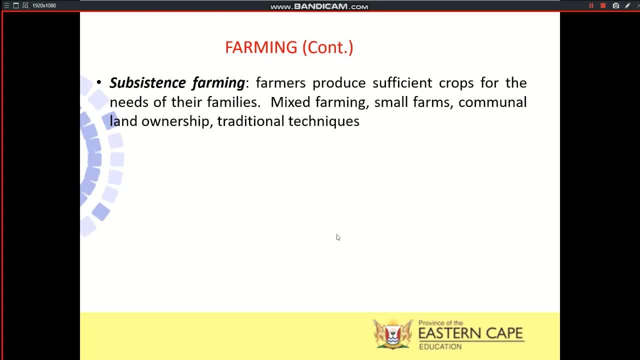 every piece of land this farmer, And it's usually small farms. There's usually communal land ownership and traditional techniques are used. This is the characteristics of subsistence farming. The next type of farming is commercial farming. It is farming that is conducted. 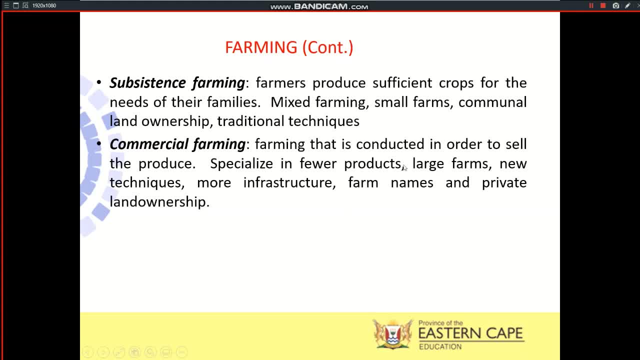 in order to sell the produce. They specialize in fewer products, large farms, new techniques, more infrastructure, farm names and private land ownership. So these two type of farming methods is very important. You must know the difference between subsistence farming and commercial farming. 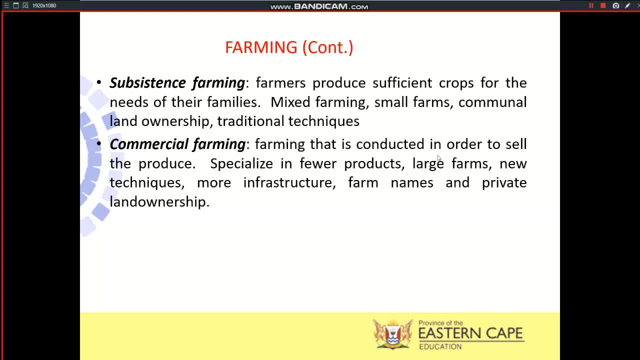 So commercial farming is a type of farming that is conducted in order to sell the produce. It specializes in fewer products, large farms, new techniques, more infrastructure, farm names and private land ownership. This is subsistence farming And commercial farming. 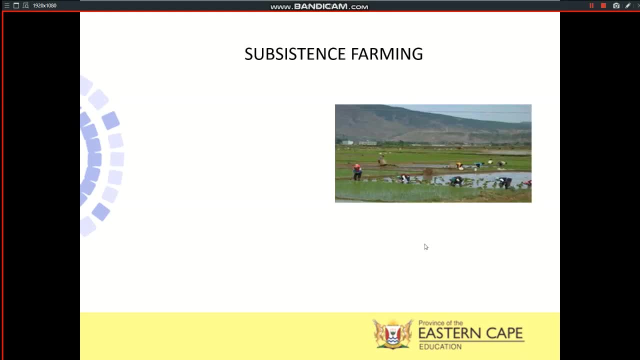 Let's look at subsistence farming closely. You see there a picture of many people farming a specific piece of land. There you find it and usually you can see many people. This is subsistence farming And you can see the crop that is usually farmed in the slabs. 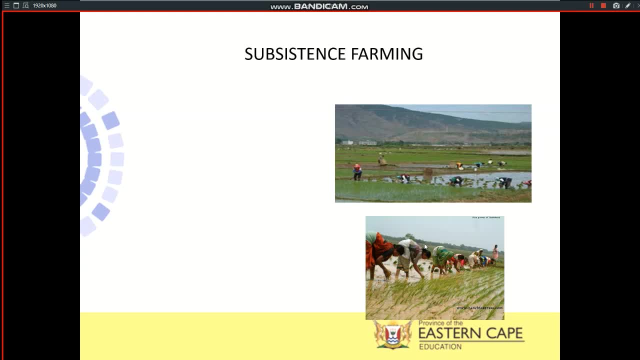 It's probably a rice pad, But you can see that it's a traditional method that is used In most instances. you see, there's no machinery with this type of farming. There's no capital involved. It's usually your cereals, rice, etc. that can be farmed. 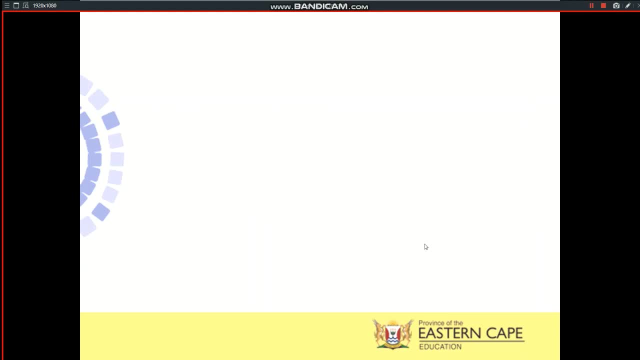 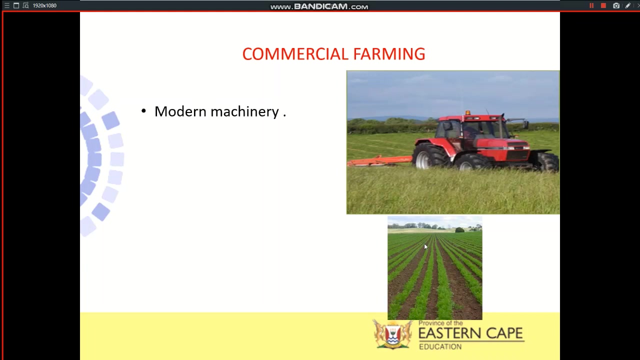 Vegetables. Then we go to commercial farming. There you have your machinery that they're showing you And you can see large tracts of land. Modern machinery is used. It specializes in certain products, It can be maize farming, etc. It's cultivating lands. 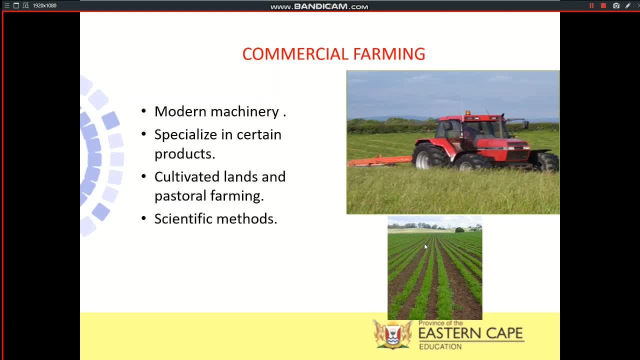 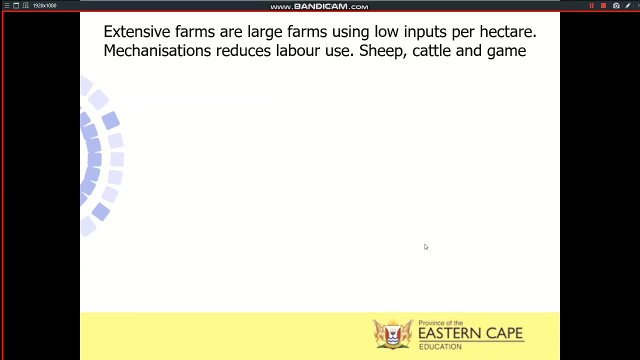 and pastoral farming And scientific methods are used, Like we basically alluded to in the previous slide. It's market orientated, In other words, it is there to make a profit, to go and sell on the market. Extensive farms are large farms. 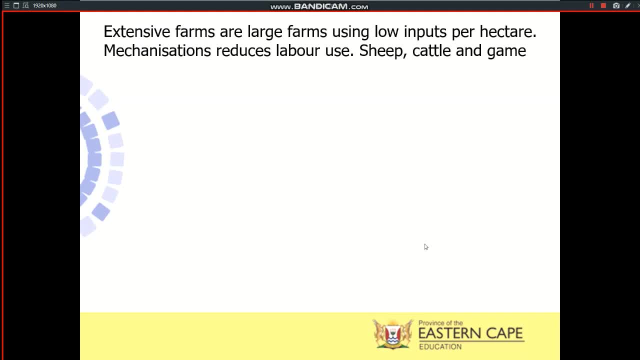 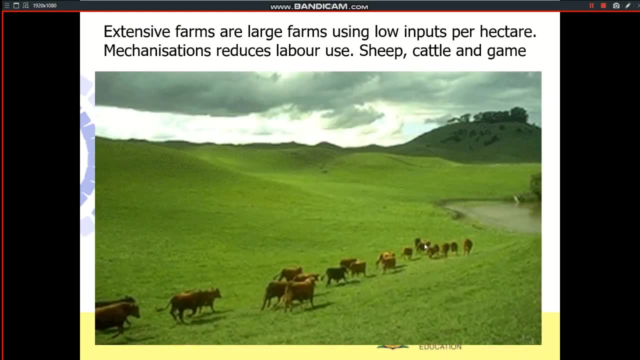 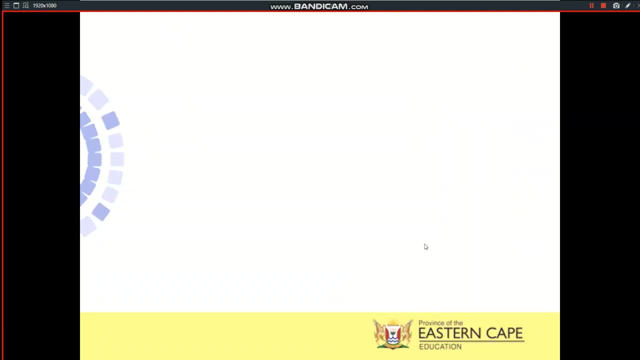 using low inputs. mechanizations reduces labor use. sheep, cattle and game farm. This is extensive farms, Right, And therefore you also need to know what we refer to as extensive farming, Intensive farming. Intensive farming is usually. 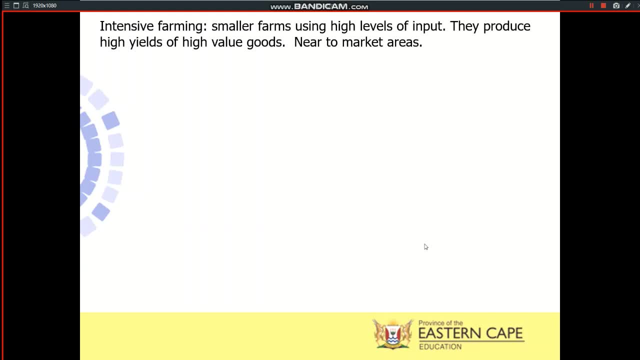 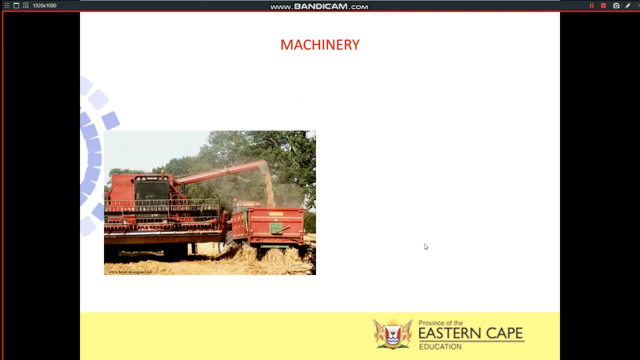 small farms using high levels of input. They produce high yields of high value goods. It's near to market areas That can be a form of intensive farming. Then the machinery. What do they contribute? Machinery is used in most instances in commercial farming. 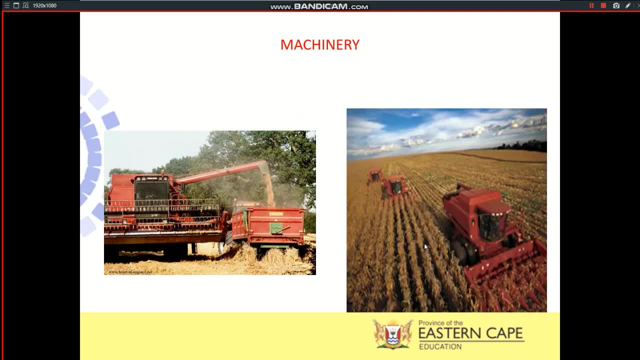 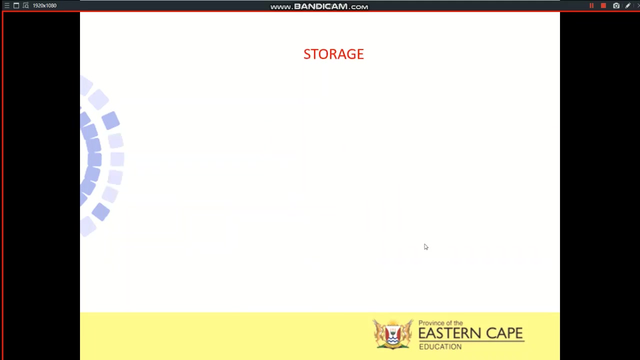 which is highly intense. There you can see large tracts of land is basically used. This is commercial farming. They use machinery and large tracts of land is farmed and most of the crop is destined for the market Storage- large storage facilities. 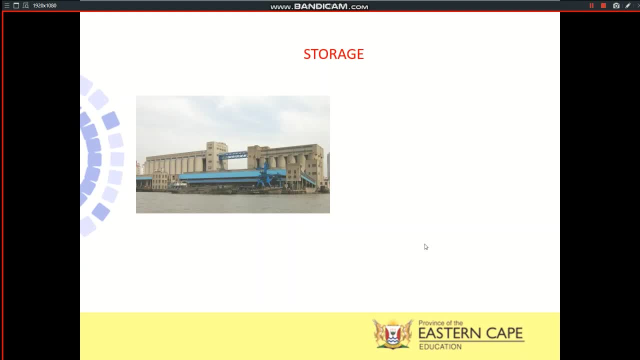 is needed for this. It's needed for this type of farming. Right And there you see silos where grain is basically stored. Right Now we come to the following: What are the factors that favor agriculture in South Africa? And this is very, very important. 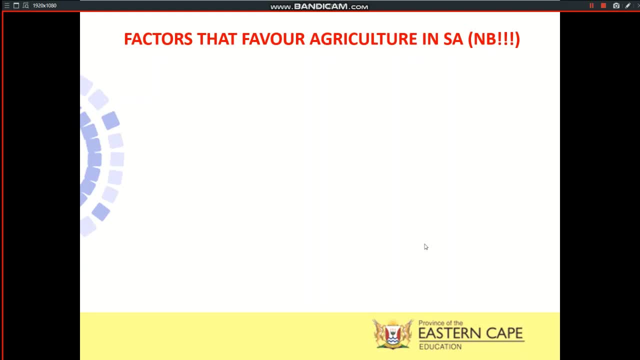 This is very important. learners, You must know the factors that favor agriculture in South Africa: Climate: You've got a favorable climate that is responsible, that favors our agriculture. A range of climates makes it possible for many products to be farmed. 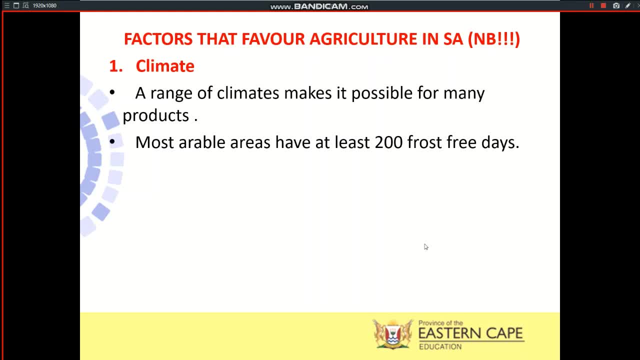 Right. Most arable areas have at least 200 frost-free days, In other words, frost does not basically influence the farming. Basically there are 200 frost-free days and because of that favorable farming it actually favors good farming conditions. Our temperatures are neither too hot. 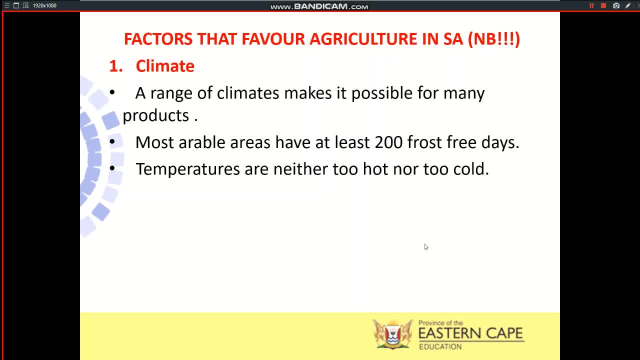 nor too cold. So it's very, very important that we have a favorable climate. Subsistence farming Farmers have developed coping methods of dealing with moderate droughts. Improved climate research has made drought prediction more accurate. So when we look at the factors, 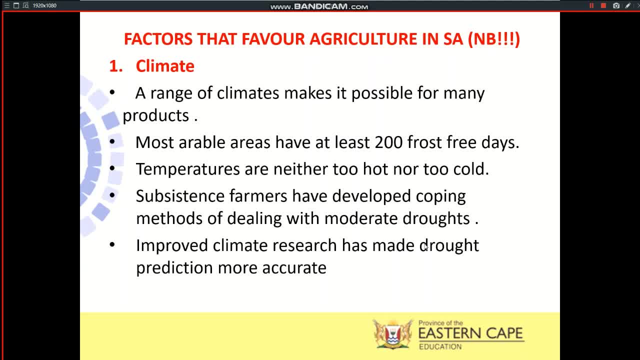 favoring agriculture. we started off with the first one: climate And under climate. these were the factors. And then our last one over here is the East Coast, Because on the East Coast we have warmer weather conditions favored by a warmer climate. 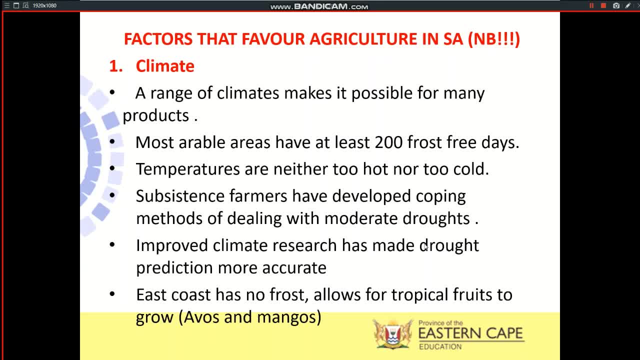 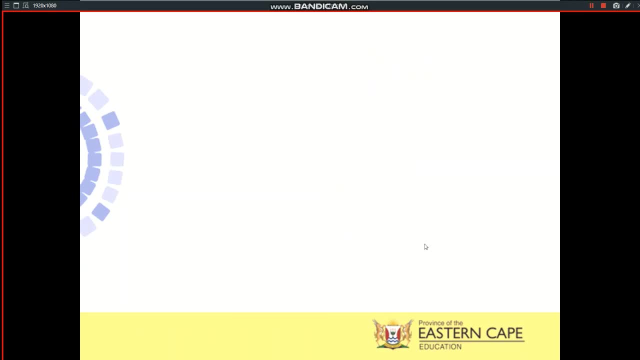 higher temperatures it allows for. it has no frost. it allows for tropical fruits to grow, such as apples and mangoes, Because of the type of climate that you have on the East Coast. There's also high rainfall on the East Coast and that favors sugarcane farming. 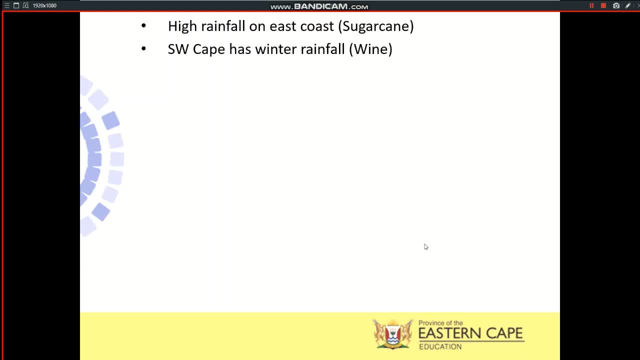 Then we have the Southwestern Cape, on the West Coast. It has a winter rainfall, A Mediterranean climate because it has a winter rainfall, And here wine is a favorable product. Rivers and lakes can supply additional water. Then we come to soils. 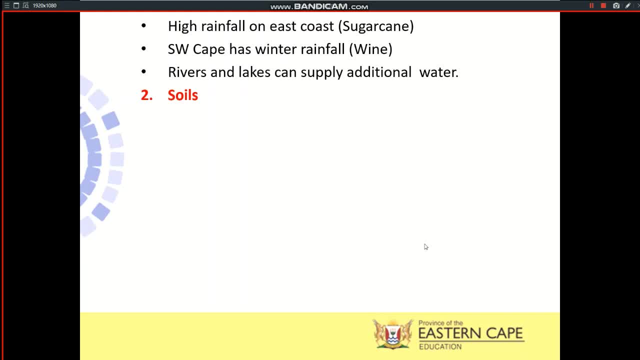 How does soil favor our farming, our agriculture? Much of the landscape where we have our products. much of the landscape is flat. That favors agriculture. Neutral soils across the country. It is suited to livestock and mixed farming. Exotic crops introduced can produce higher yields. 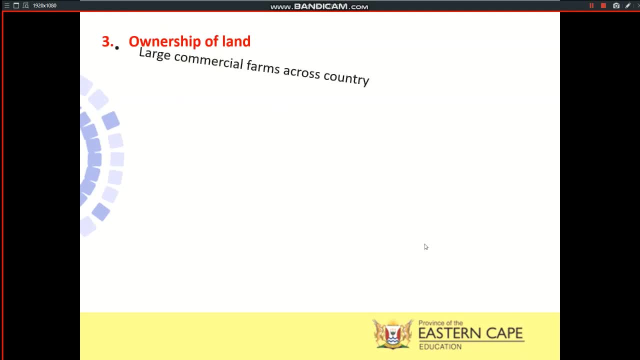 Let us look at ownership of land: Large commercial farms across the country. We have a number of large commercial farms across the country: Irrigation, watering of crops, Genetically modified crops and pesticides- It's found here. water from transfer schemes. 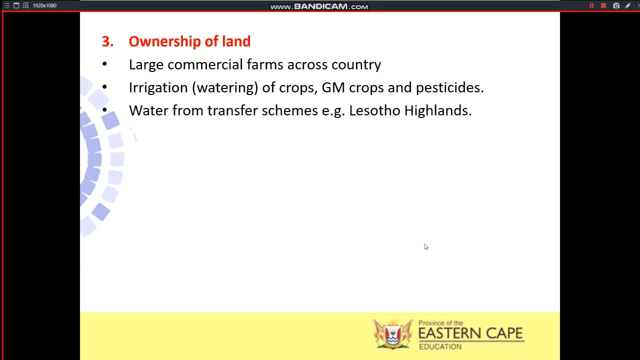 Example is the Lesotho Islands scheme. Trade: The European Union and South Africa have no trade restrictions. Import duties are limited. The Northern Hemisphere relies on South African products in the winter, In other words wool. And just to make learners aware, 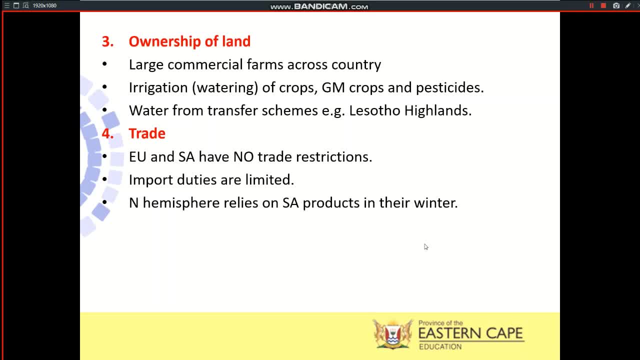 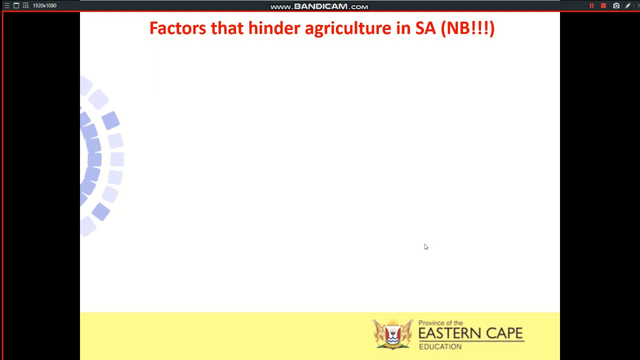 with wool. the largest producers are in the Southern Hemisphere And the largest consumers of wool are in the Northern Hemisphere. Factors that hinder, in other words, factors that don't favor agriculture in South Africa: Learners, please. NB. very important. 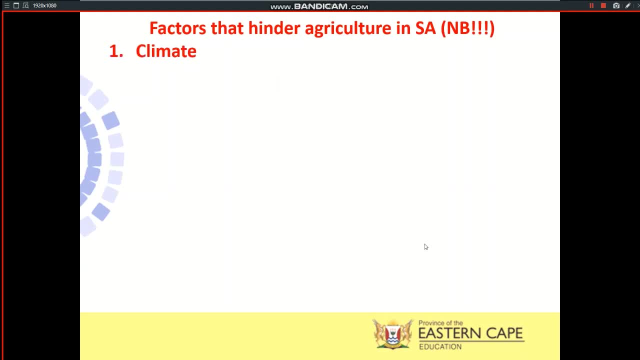 Again, let's look at the climate. We do have a situation where, in some seasons, we had drought conditions. An example is the drought that we had a year or two ago in the Southwestern Cape and that had a drastic effect on the agricultural sector. 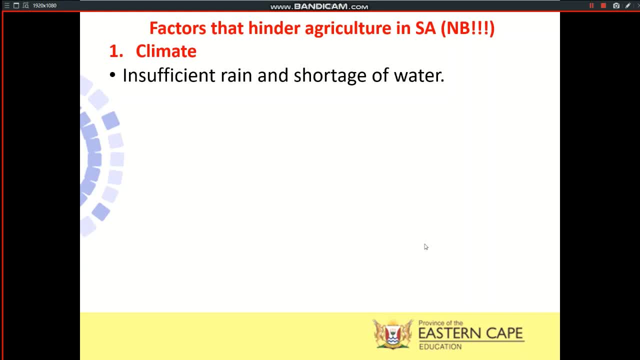 the Western Cape. At the present moment, we also have droughts in parts of the Eastern Cape as well, and this has definitely had an impact on the agricultural sector in these areas. South Africa's rainfall- annual rainfall- is 495 millimeters per year, and the world average is 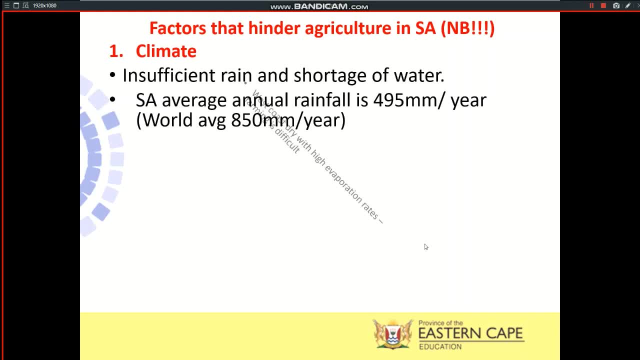 actually 850 millimeters of per year. West Coast, our West Coast, is dry, with high evaporation rates, and farming is difficult. Frost is common on our plateau. subsistence farmers are at risk of droughts, which I have already explained to you. 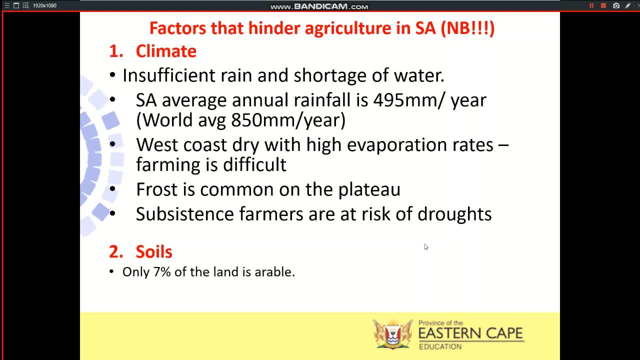 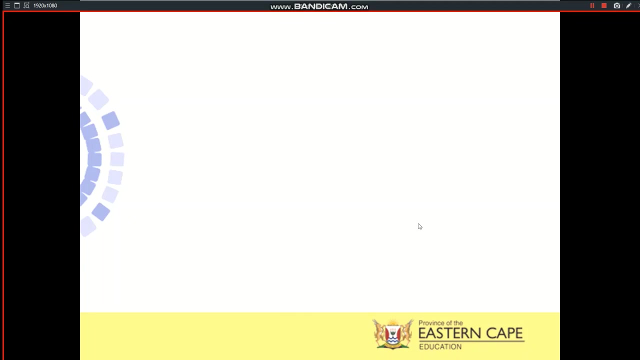 The soils in terms. only 7% of the land is arable. Only 7% of the land is arable. Many arable areas are too densely populated for farmers to develop commercial farms. Soils are thin, especially those on steep slopes. Alkaline pH is greater than 7.. The 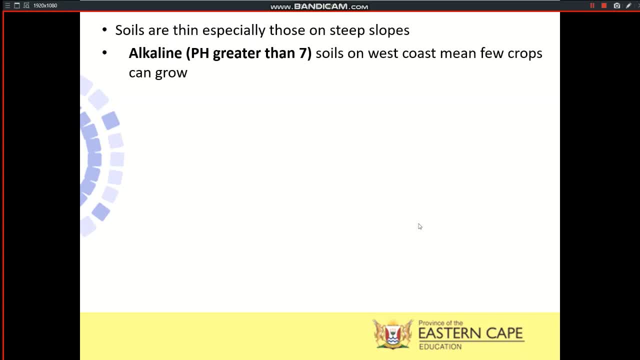 soils on the West Coast. both mean fewer crops can grow, So we are over grazing and poor farming techniques has damaged soils. Some of our exotic crops, like maize, produce good yields in years with enough rain, but it can be very poor in times of drought, which I have already. 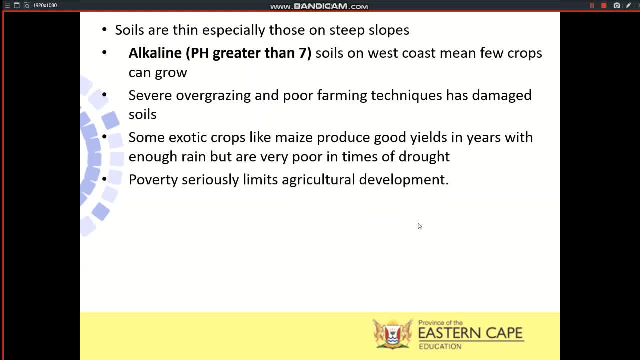 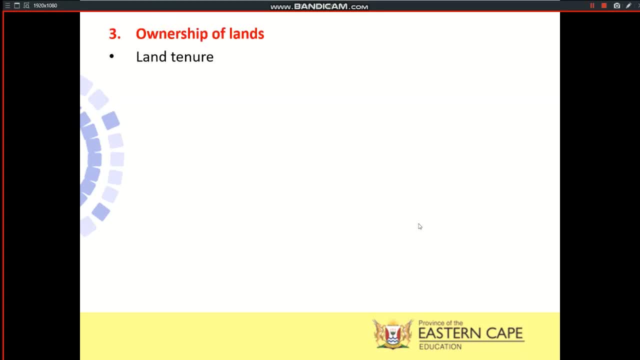 alluded to- Poverty seriously limits agricultural development. The ownership of land- we have a problem with land tenure which we already spoke to you about- under Settlement Geography Nationalization, Farmer tax which is becoming common in South Africa. Then trade Subsidies after 1980 decreased. 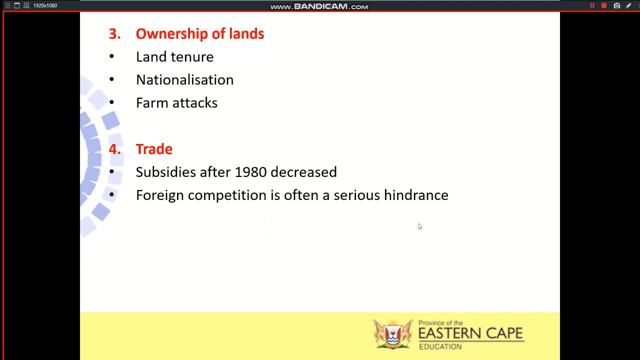 Foreign competition is often a serious hindrance. Fluctuation in maize price has hurt farmers. Now we come to a very important aspect, and this is food security. Learners, you need to know what is the definition of food security, When it means when all. 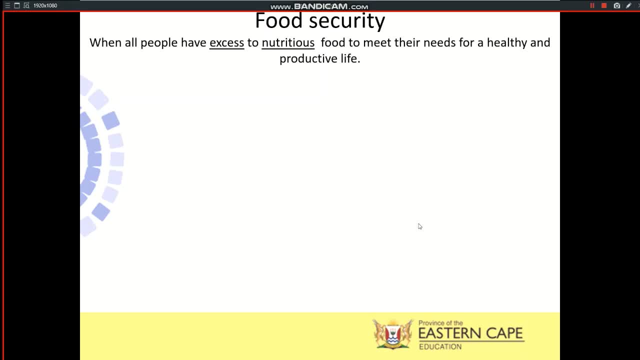 people have access to nutritious food to meet their needs for a healthy and productive life. This means if everybody- everybody- should have food security. this means if everybody should have food security. This means if everybody should have food- enough food that is nutritious for them to be able to have a healthy and productive life. 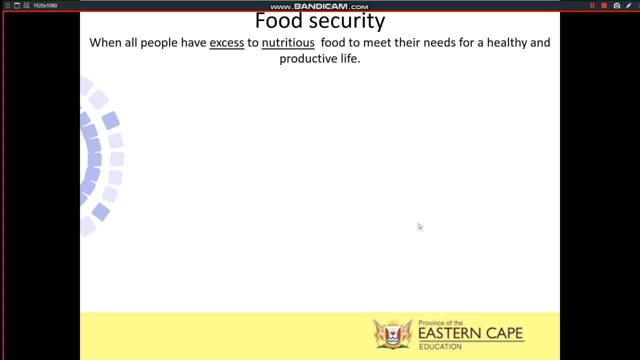 And that is what we call food security. What is food security and how does it basically contribute to our country and basically to people? Food insecurity is the opposite of food security. It exists when people live in fear of hunger and starvation. It's basically when people are hungry. 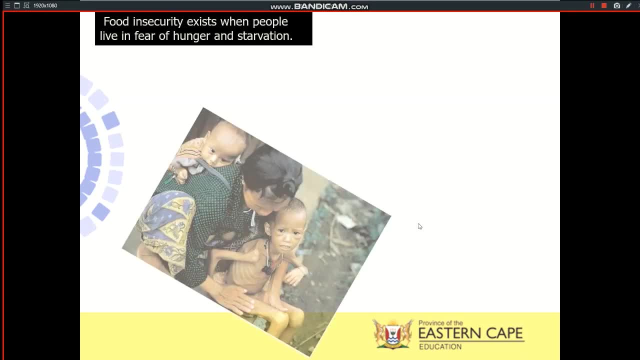 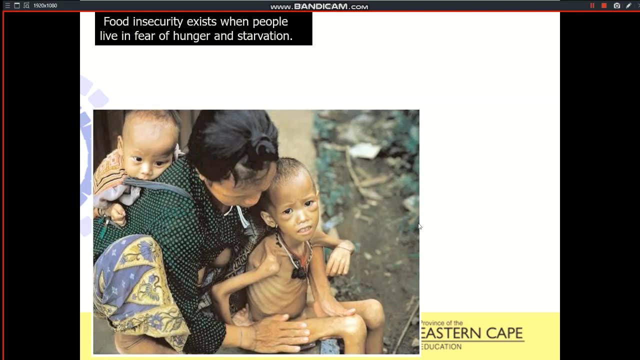 And the starvation exists. That is basically what you see in countries, especially where we have problems such as malnutrition as well. As many as 39% of our population in our country lives with food insecurity- This is a reality- And lives with food insecurity. 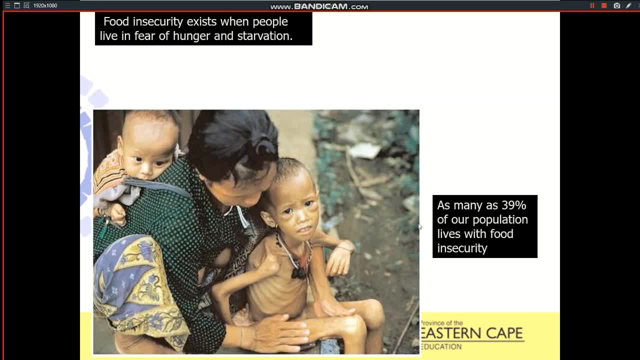 Learners. you need to go to your newspapers, You need to go to the internet And you can actually go and research up on food security and food insecurity And look at it in the world and specifically in your country And see how has this affected people's lives. 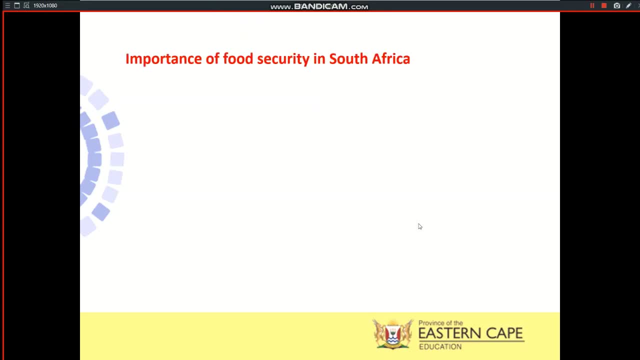 What is the importance of food security in South Africa? Food needs to be available on a national and a household level Means our farmers must be able to produce enough food so that people can buy food and have it readily available for consumption. Foods must be accessible on a sustainable basis. 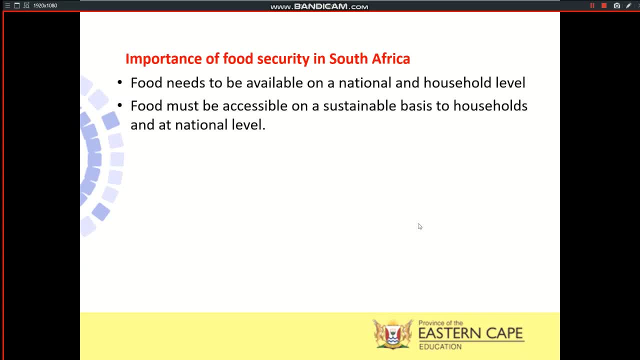 Foods must be accessible on a sustainable basis to households and at national level. It means that number one: it must be accessible and sustainable. It must be there continuously for households and at national level. Foods must also be affordable. Food supply must be reliable and produced under safety. 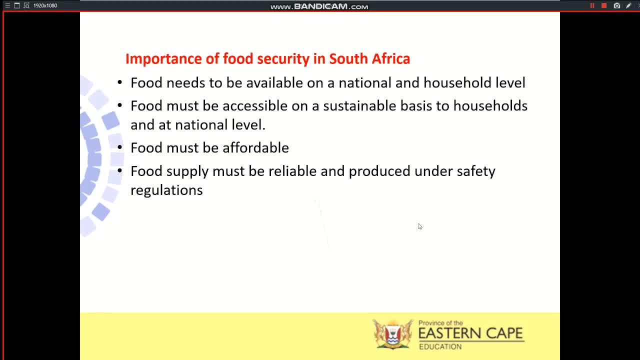 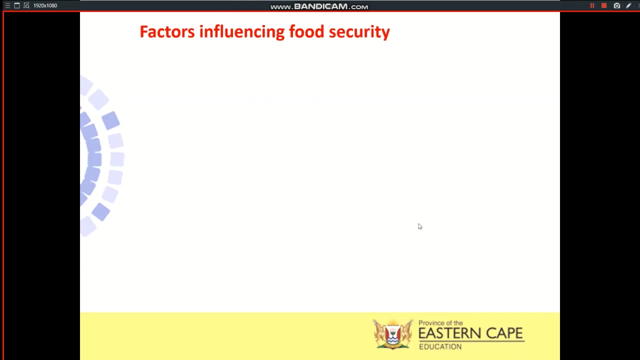 Food safety regulations. Food must be distributed so that the country is food secure in all areas. What is the factors? what are the factors that influence food security in our country? Climate effects, such as floods or droughts. We've spoken about floods or droughts already. 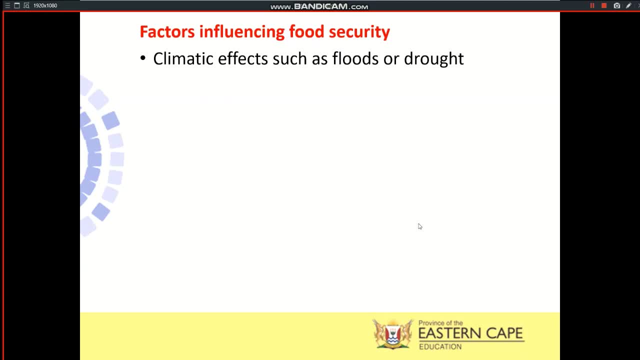 And you've also learnt about floods and droughts. You went through the specific aspects. You went through this in your grade 11 syllabus as well. High fuel prices makes food products more expensive to transport. High levels of HIV AIDS lowers productivity and yields. 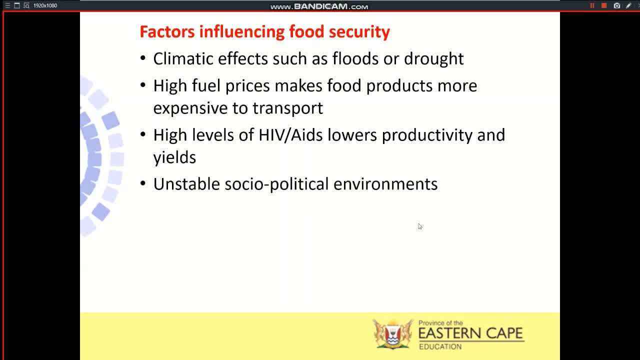 There's unstable socio-political environments, which threatens our food security. Imbalances in trade means that consumers push prices. Lack of natural resources hampers their ability to produce. Lack of the ability to grow food: Population grow. As population grows, so must foods supply. 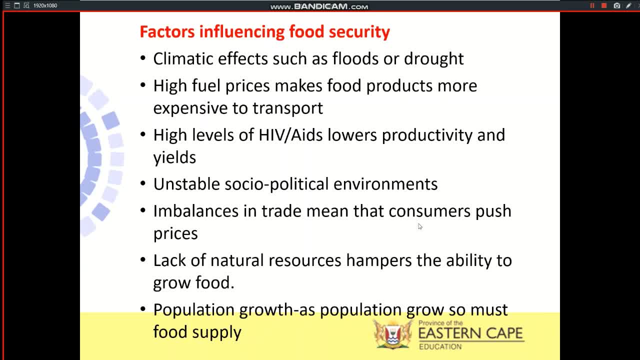 Now just to say something about our factors influencing food security. If you look at all these factors, learners, it is basically factors that you can actually apply to your present context That you are living in our country. Read your newspapers and see how you can actually apply these factors in the present situation we find ourselves in. 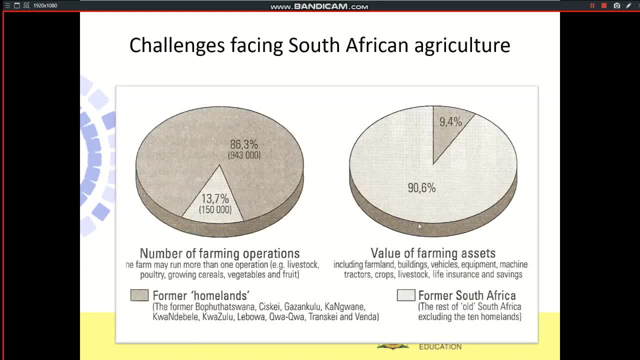 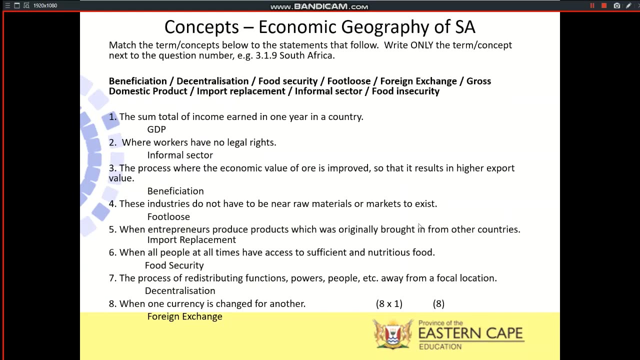 Related to your context. Let's look at challenges facing South African agriculture again. We've gone through them already, So we won't be going through them again. You have done them in the previous slides. Now we're going to look at how this section is basically. how can it be asked in the exams? 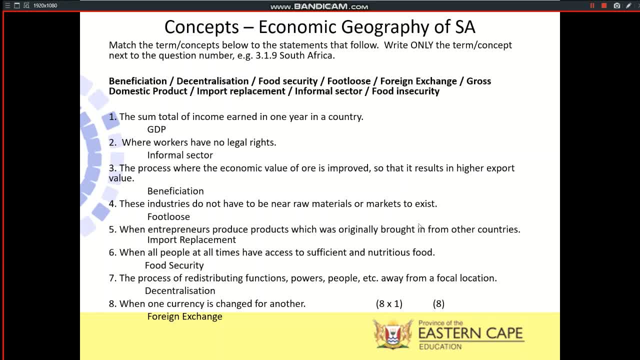 We look at an example. It's been taken from a previous question paper where they actually examined or tested your concepts, And it can be asked in the following way. They asked the following examiners: It was examined in the following way: The sum total of income earned in one year in a country. 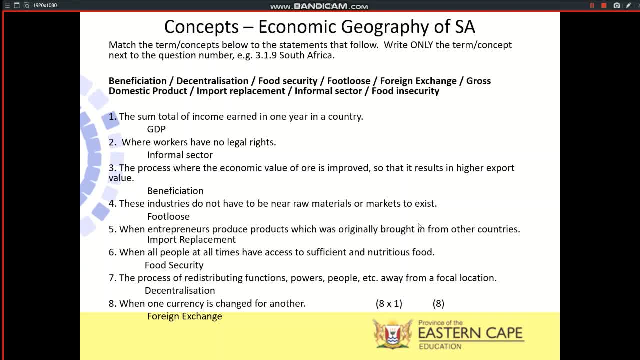 They speak of the GDP. So you had to go to the concepts. They give you all the concepts And you need to relate the concepts And then you need to give statements from the terms below And you might need to match it to that. 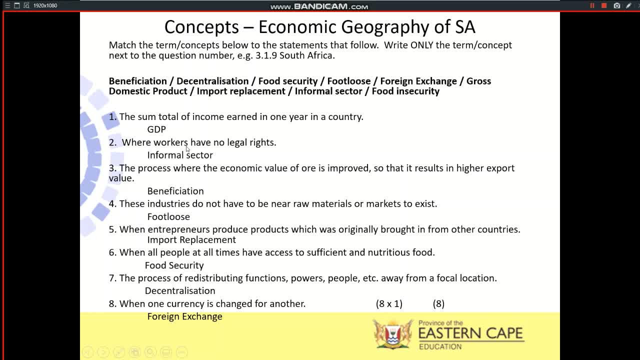 Where workers have no legal rights. That's the informal sector, The process where the economic value of oil is improved so that it results in higher export value Beneficiation. These industries do not have to be near raw materials or markets to exist. 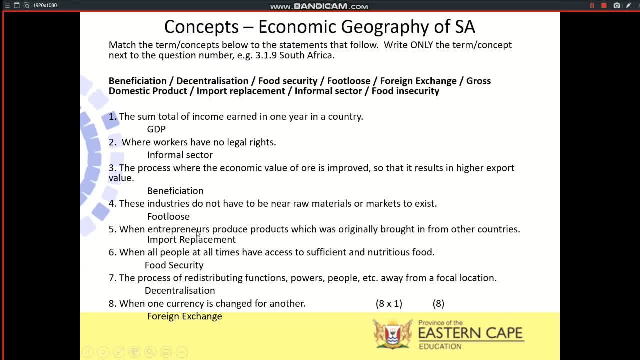 It's called footloose industries, When entrepreneurs produce products which are originally bought in from other countries, Import replacements, When all people at all times have access to sufficient and nutritious food, We call that food security. The process of redistribution of functions powers people away from a focal location. 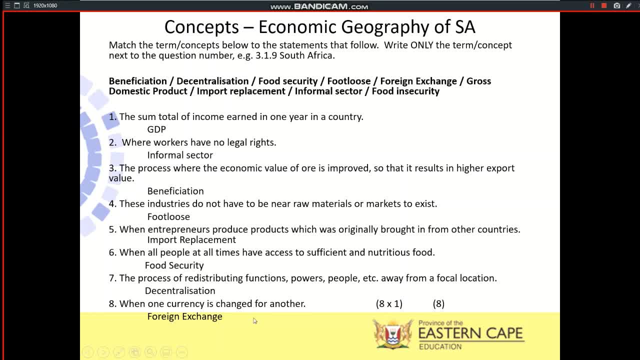 It's decentralization. When one currency is changed for another, That is called foreign exchange. This is just an example Of the way in which your concepts can be asked, And it counts eight marks, So it's important that you know your concepts. 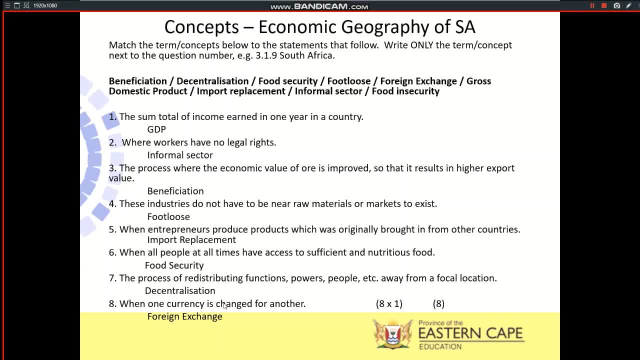 Like I've already told you what to do, And go through question papers and see if you can find these type of questions, Not only for this section but for all your other sections. Go And see what type of questions you can get. that is similar to this. 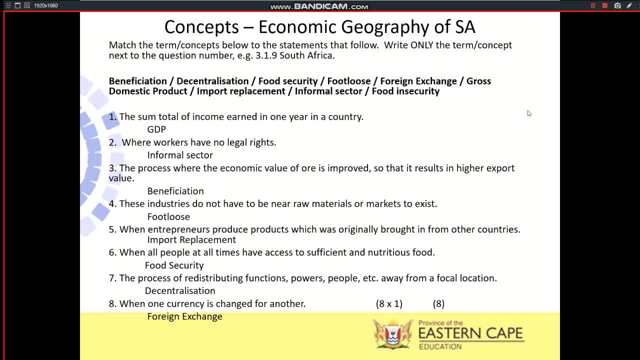 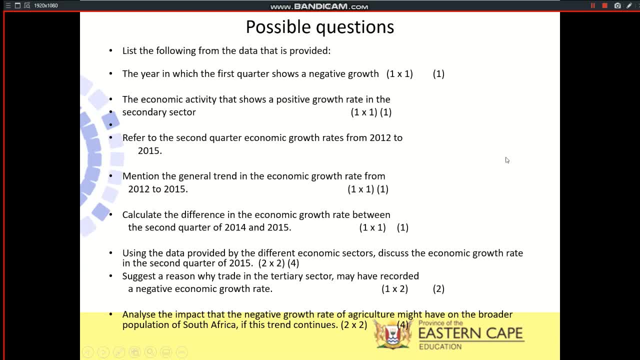 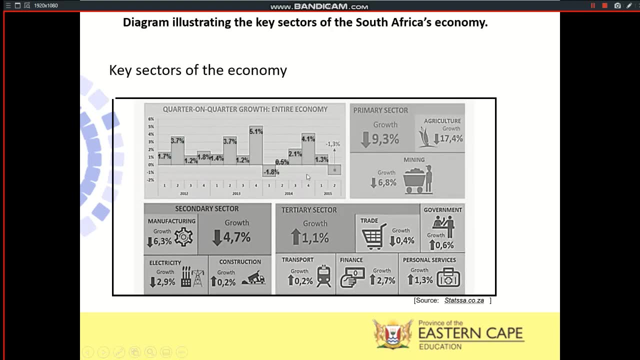 And you'll see how easy marks are scored. Our next section that we're going to do, In other words, the next possible questions, Or the next way in which questions can be asked is. This is taken also from a previous question paper. Here again, they give you a diagram. 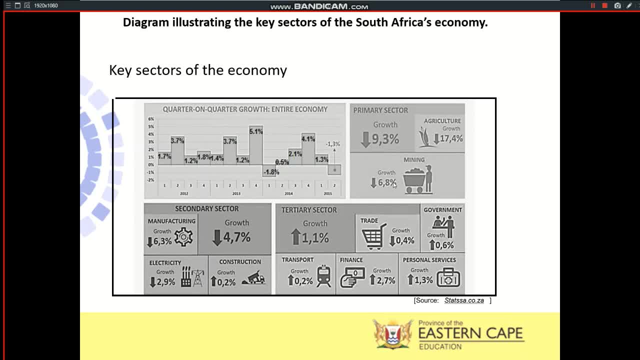 Which illustrates The key sectors of the South African economy. And here you can see, they give you bar graphs And they give you information. And this is a graph, Or let us say this is a diagram, Where they give you a lot of information. 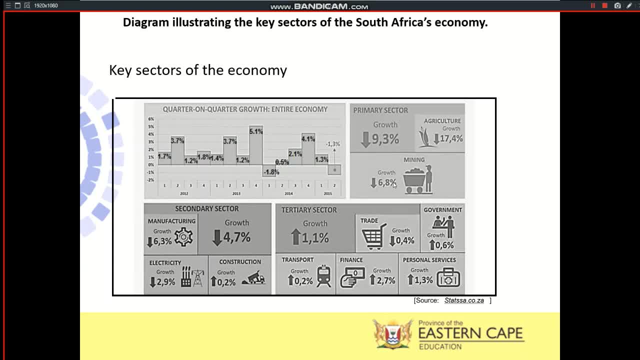 They're giving you bar graphs, They're giving you percentages. They're actually giving you also The different key sectors of the economy. Let's look at them. They give you In one part of the diagram It's quarter on quarter growth. 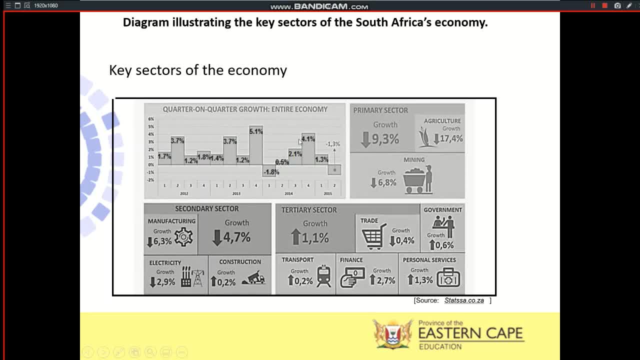 For the entire economy. So they give you the quarters For the different years Right For 2012,, 2013,, 2014, 2015.. They give you another part of the diagram. Diagram is The primary sector. 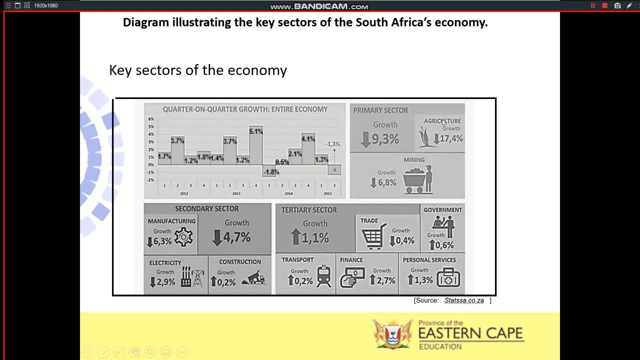 Growth: Agriculture Growth, Mining Growth. They go to the secondary sector- Manufacturing, Electricity, Construction, And it gives its growth. They go to the tertiary sector: Transport, Finance, Personal services, Government Trade And its growth. 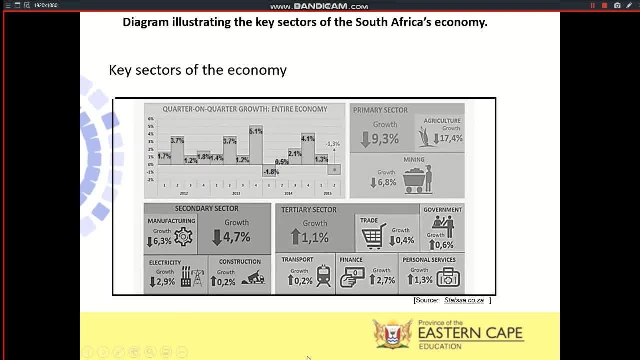 So Here you can find a typical example Of a diagram That illustrates the key- illustrating key structures of the economy. Let's look at the questions that they can possibly ask on this diagram. They say: list the following from the data that is provided: 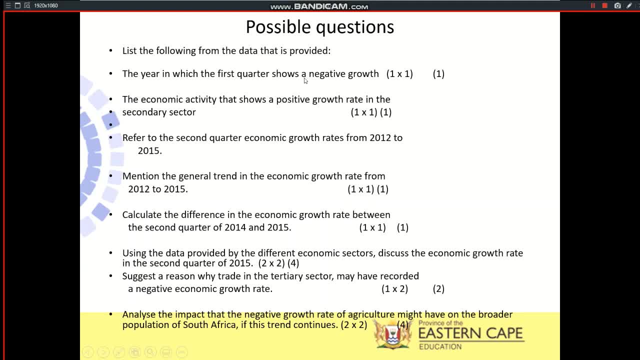 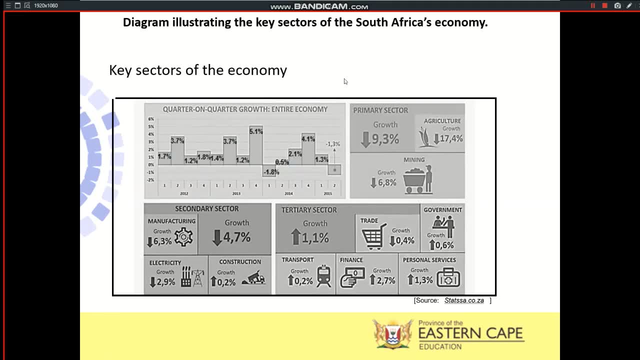 It says The year in which the first quarter Shows a negative growth. So if we go to the diagram And it says the year, the first quarter, Yeah, Here's the first quarter of 2014.. This is the first quarter. 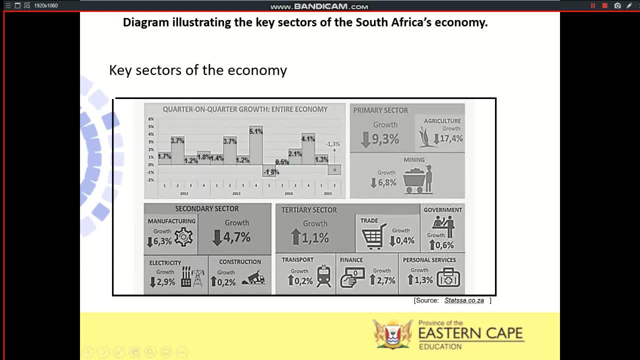 You can see it showed a Minus 1.8% growth If you compare to the other Quarters. So in 2014, the first quarter Showed that- That That growth. So It means you need to. 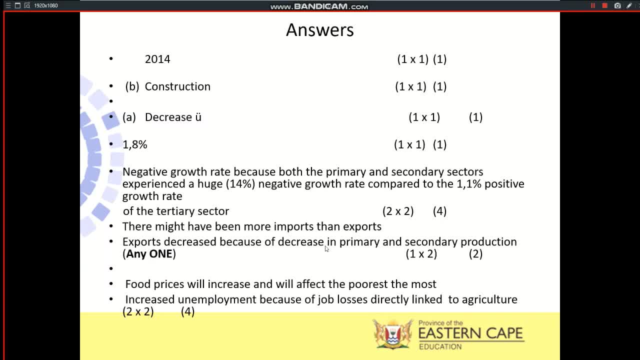 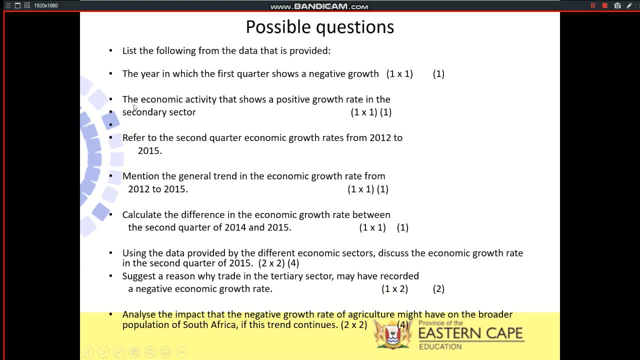 Study The diagram Carefully: The year in which the first quarter, that. then it says The economic Activity That shows A positive growth In the secondary Activity, Then it goes on If you go to the secondary Here. 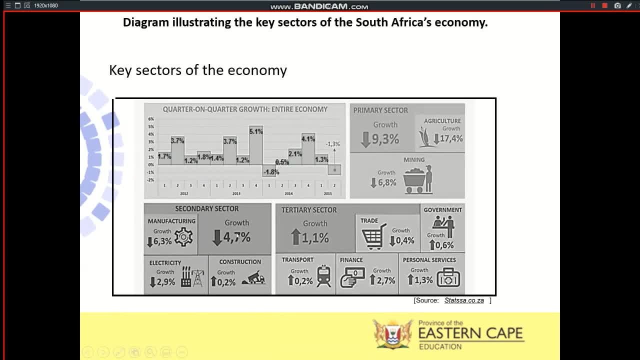 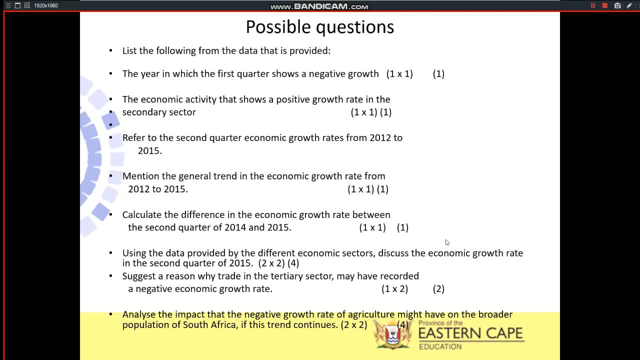 We go to the secondary Activity. Yeah, And the question It's Asked Was The Economic Activity That shows A positive Growth In the secondary, Secondary Sector. So if you go to the secondary sector, 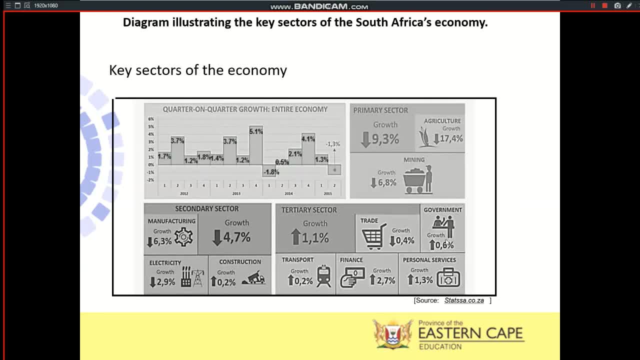 Which one showed a positive Growth. We should go through all of them. It was Manufacturing. So If you go to the Secondary Sector, Which one showed a positive Growth? Then It says: Refer to the Second. 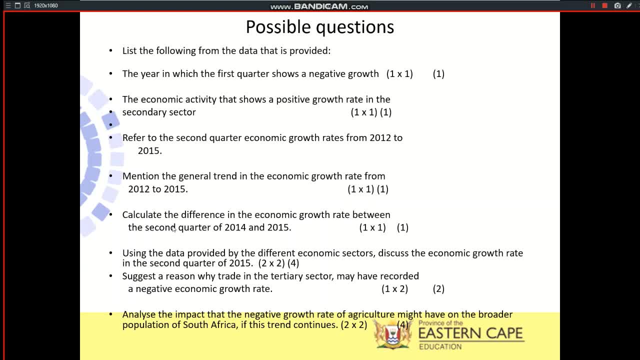 Quarter Economic Growth From 2012. To 2015.. Mention The General Trend In The Economic Growth From 2012. To 2015.. And, If You 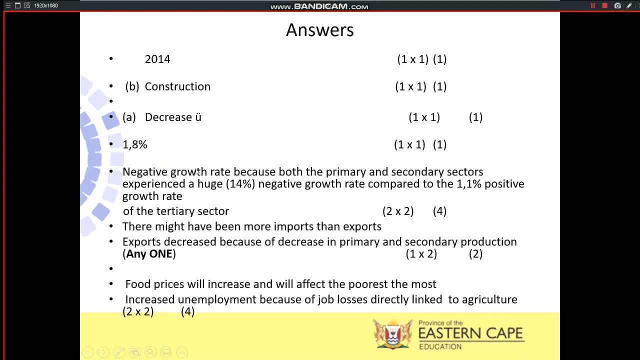 Look At This. It Goes For The Primary And The Secondary Sectors- Experienced A Huge 14% Negative Growth Compared To The 1% 1.1%. 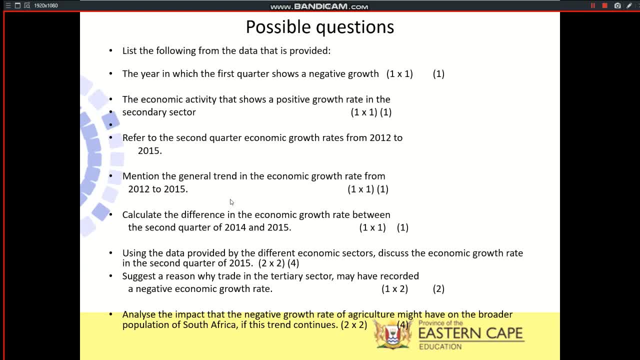 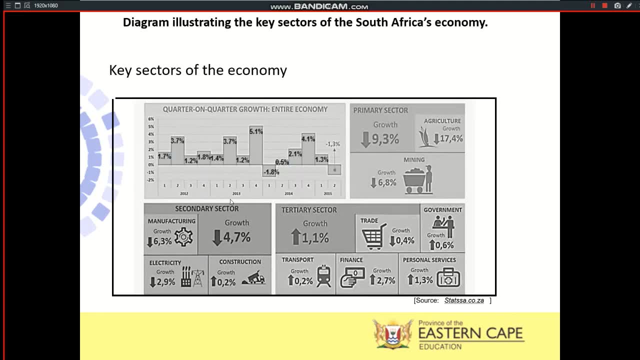 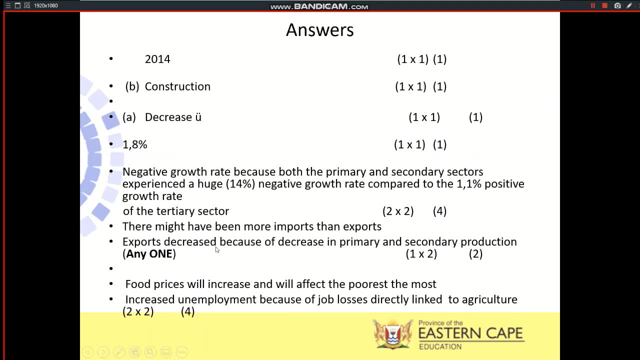 Positive Growth Rate Of The Treasury Sector Right The Next, The Secondary Of The Economic Growth From 2015.. To 2015.. It Gives You The 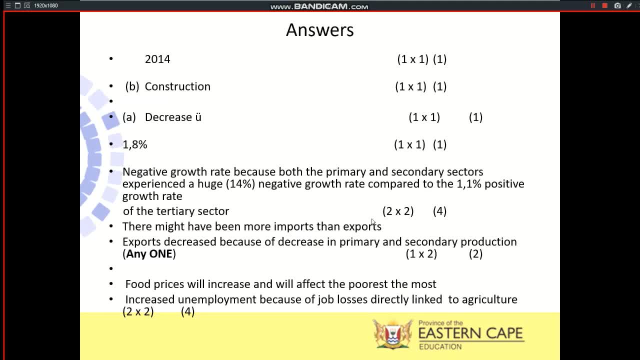 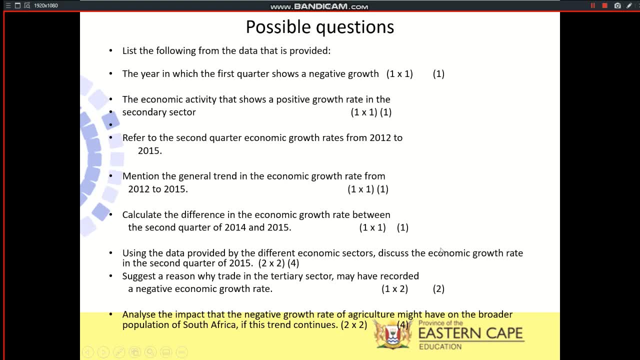 Following. If You Look At It, Might Be More Imports Than Exports If You Calculated. It Suggest A Reason Why Trade In The Treasury. 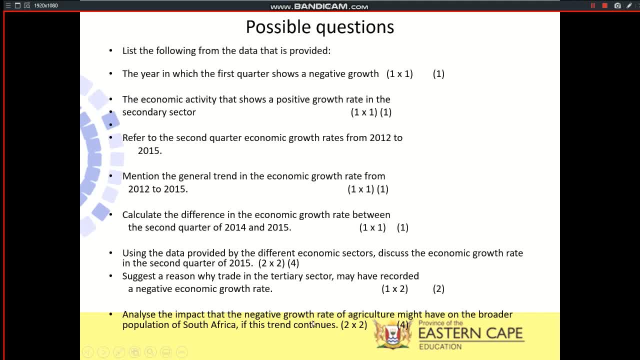 Sector May Have Been Recorded As A Negative Economic Growth Rate. Analyze The Impact Of The Negative Growth Rate Of Agriculture Might Have In This.